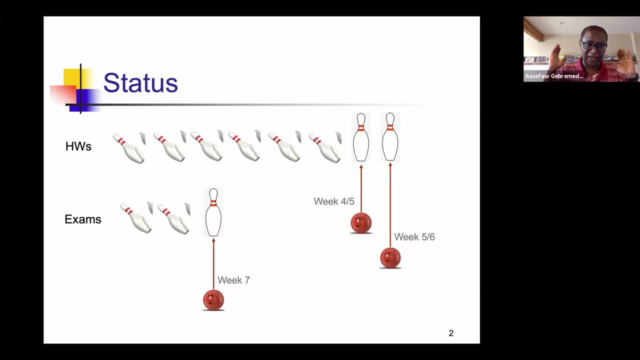 knocked down quite a few things, So we've got six of our eight homeworks. So we've got six of our eight homeworks done and two of the midterms done, And so we are left with the finals. And then we've got two homeworks left, And what you see here in this picture is: 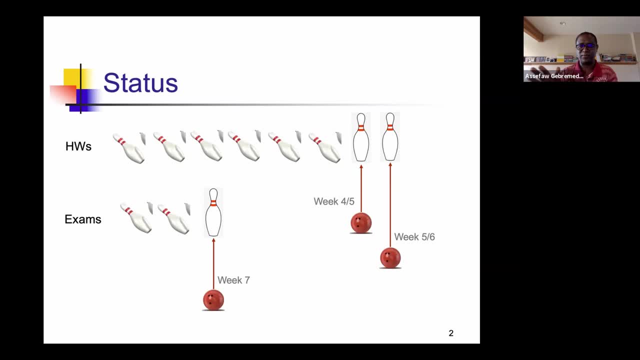 what we have accomplished and what is remaining and what times they will be done. And so this week is week four and we will have our seventh homework out, And I'll ask you whether you still want it on a Friday. I probably would have wanted it on a Wednesday to go out, but let's say it's going to go out on a Friday. 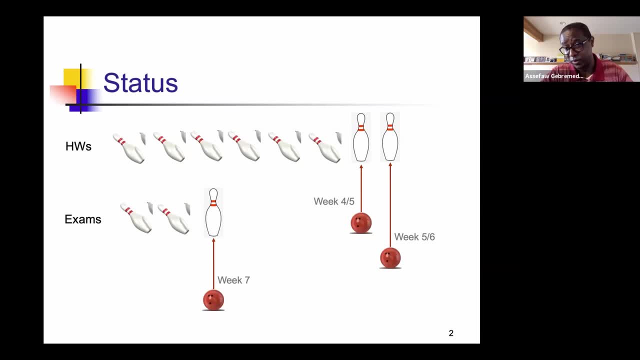 this week and it will come in next week. That will be week five, And then in week five, as you give me homework seven, you get the last homework, homework eight, and that will be due in dead week, and that will be week six, and the final will be, of course, in the finals week. And so this is where we are headed. Here's what we have accomplished. I thought bowling would be a good way to show this, and- and this is my attempt to showing you how this 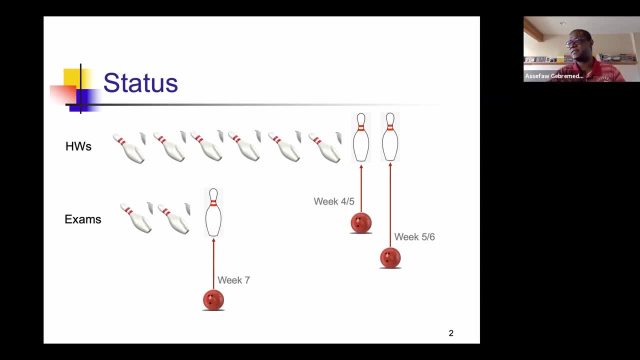 has unfolded so far, So. so I'm going to use this time to just use this as an excuse to get our warm up question a little delayed today. So so now you see here bowling, and I'm not sure how many of you are bowlers, but I want to know. 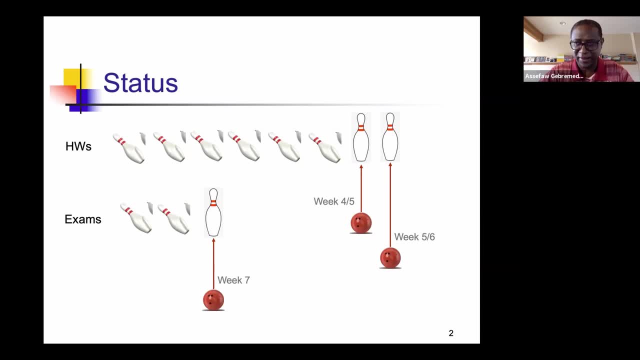 what your favorite sport to play is. And we'll get started with the topic we have for today, And it is a new topic that will equip us with more things, to you know, under our belt to get a come, you know, to get to get working with around theory of computation. but let's 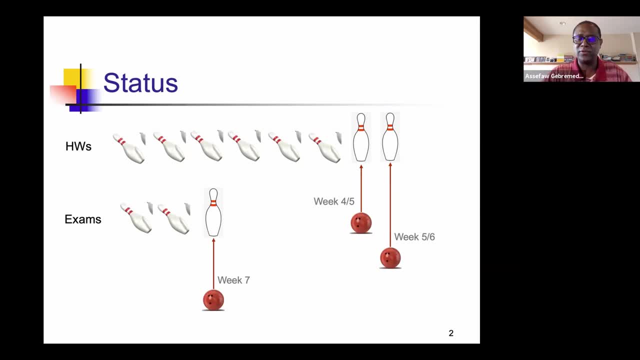 because we have this slide up, Let me hear from you what your favorite. So that's warm up question. Warm up question number one for the day: What, and probably will be the single question- What is your favorite sport to play? You go ahead and give me. For those of you who can't make up your minds between two things, I will allow you to give me two. but a favorite sport to play- Bowling- counts as a sport, in case you wondered. Well, go ahead and tell me what it is that you 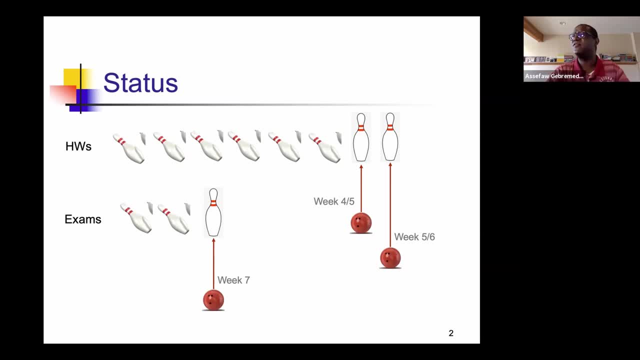 think is your favorite sport to play. I'll give you a second for those who are struggling with my WSU to join. This will be a good excuse for them also, And so let me, let me hear from you for 30 seconds, about a minute or so, to get going there. And once again, congratulations on having. 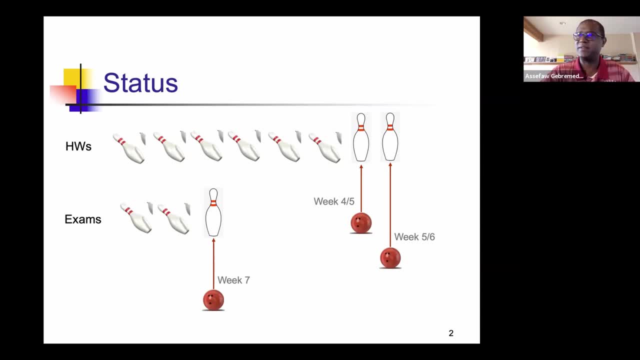 midterm, two behind you and I'll ask you how it went. Maybe. maybe you will tell me. in general I have kind of, we are going to grade and you will hear back as soon as I finish grading. but I have picked a little bit and then just to get a sense, and I've seen a few and from the few that I have seen it looked like you should be good and they were all good submissions that I have seen. but we have to carefully grade it and you will hear back from me. So 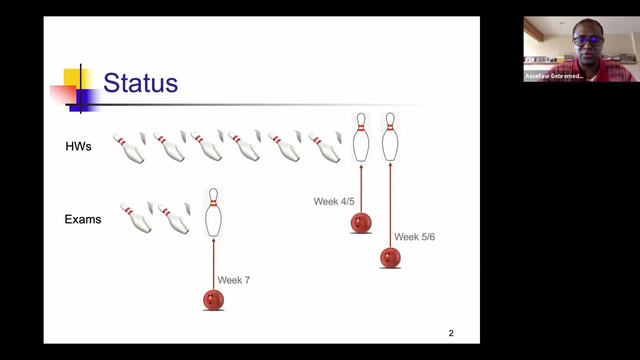 warm up question is: what is your favorite sport to play? and you are giving me some very interesting answers and you will get back from me when I start looking at these responses later on. If we have given me enough for that one, I'll turn the question a little bit around and ask you: what is your favorite sport to watch? So to play was whatever you have told me. now The second question is to watch, and I will know what the distinction has happened. 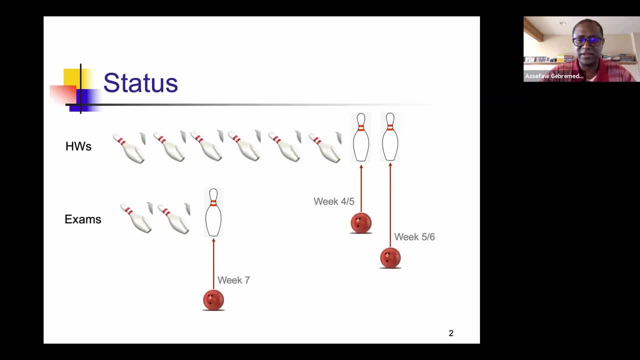 By the answer you would give me. But if you want to qualify it, you would say to watch, and then you say: whatever it is So to play and to watch. There may be some people who would enjoy playing the same sport that they watch, and there will be some people who would watch something else. 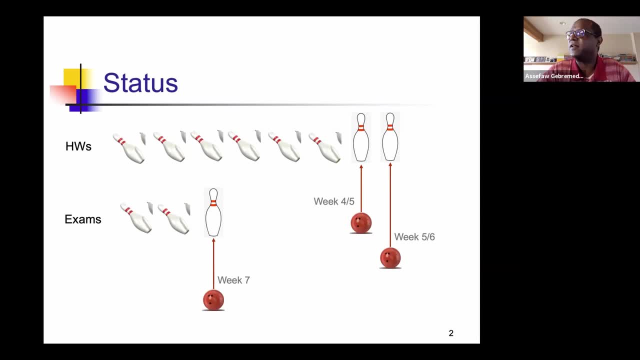 Enjoy something else, And when it comes to playing, they would play something else. So so, favorite to play was the first question. Now you say favorite to watch, as To watch, Exactly. And then for the second ask. for, if you are kind, you can tell me that you're now responding to that by telling me that, if you are responding to the question on watching, 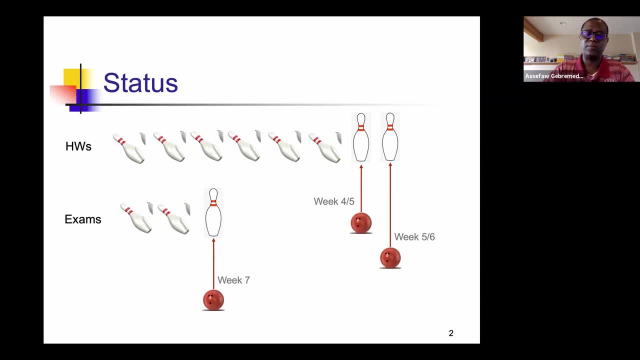 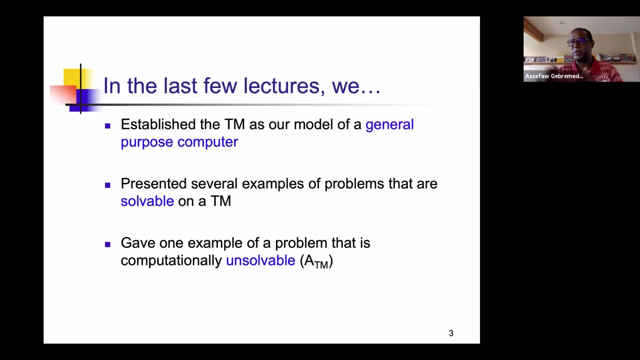 Alright. so this I cheated. I said I'll give you one Warm up question, but there were to go ahead and give me those and we'll get started in a second with today's topic. Alright, keep, keep answering those and they should come in, and then we are having more people to join us. We start, let me get going, And then I'm going to start with what we've done so far and what we'll be doing today. 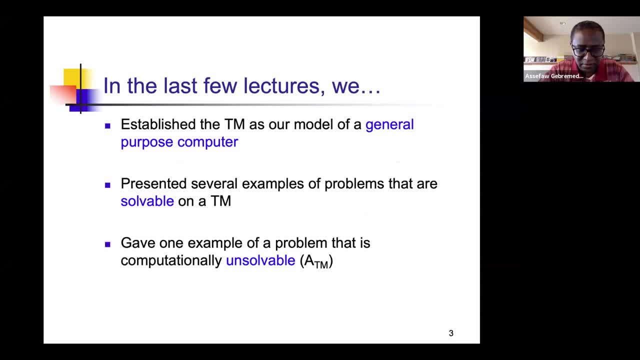 So in the last Few lectures- If you've seen what we did, especially after spring break- we spent quite some time talking about Turing machines in general. Turing machines in general- and we made the case that these are- is our model for a general purpose computer, and then we made a series of 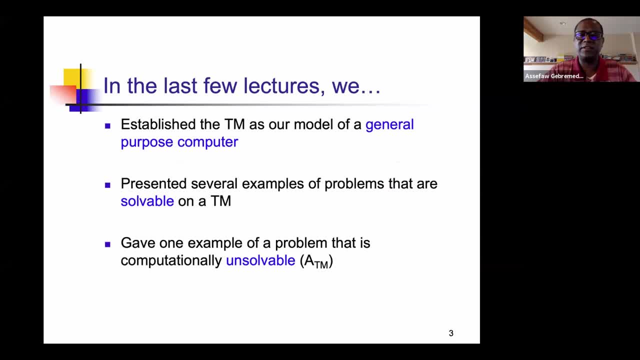 You know founding matters around it that would establish that this is in fact powerful enough to be considered to do what the general purpose computer Do. If you look at what we did in Chapter four of the book, The last three, four lectures, we first looked at problems that are sold on the Turing machine. We discovered that there are some problems that are not sold. 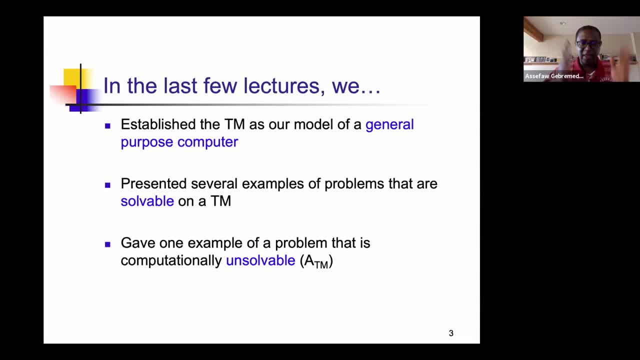 But there were some problems that are sold on a Turing machine. So we have given a precise definition for when to say a problem is algorithmically solvable, And so we looked a long list, Quite a bit of a list, And we went through. 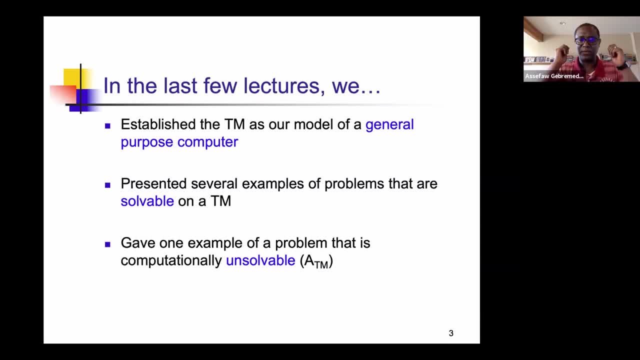 formally giving evidence for the fact that these are solvable by exhibiting a Turing machine that we decided. If you look at the last two, three lectures we had, they were on unsolvable problems and we first of all said what it is and then looked at Hilbert's tense problem and introduced the technique for swing. but 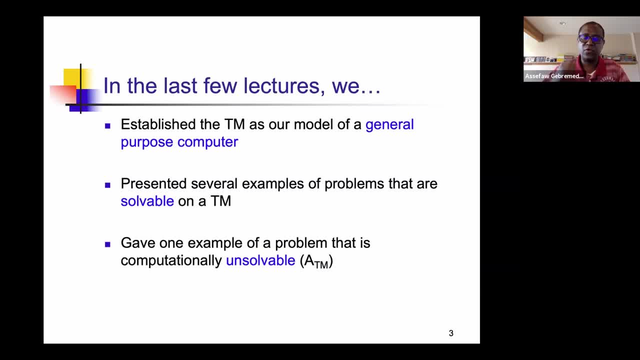 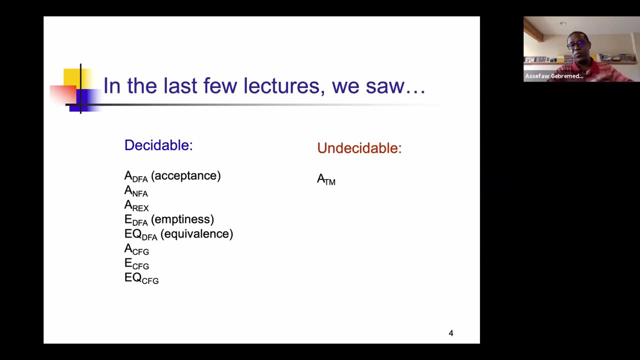 there was one problem on which we spent almost two lectures and formally showed that it is unsolvable, and that was the acceptance problem on a Turing machine and we called that problem ATM. So we saw only one, and and that is where we kind of were in the last few lectures. If we were to group the universe that we have, 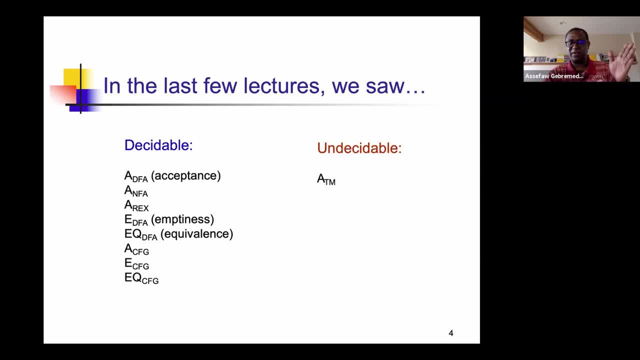 seen so far into two. we saw a very long, well, a substantially long- list of language that are decidable. so we started with things that are defined around finite automata, deterministic finite automata, non-deterministic finite automata, and, and the same kind of class could also be. 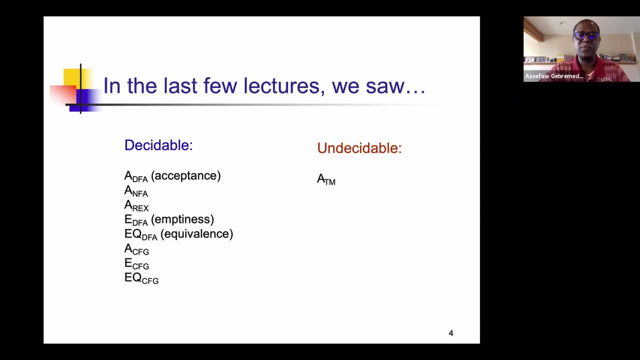 explained. So equivalence is a very common phenomenon that can be used to explain equations that are expressed using regular expressions. And in all of these cases, when we're given that model, the computing machine- and whether it accepts something or not, the A is for acceptance. all of these problems were 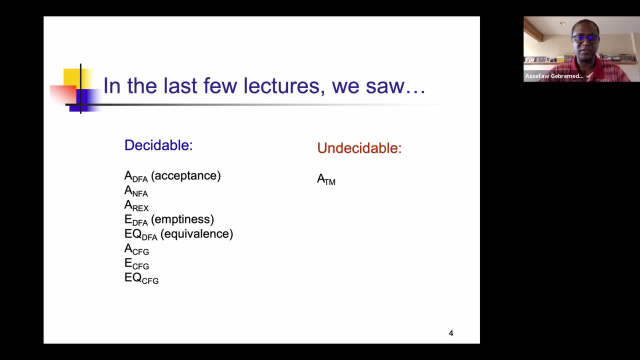 decidable. We also looked at a problem that would say: here I have a DFA, does this language, is it empty? and then? so that was an E- DFA is what we called it. We took two languages and show whether they were equivalent in DFA's and 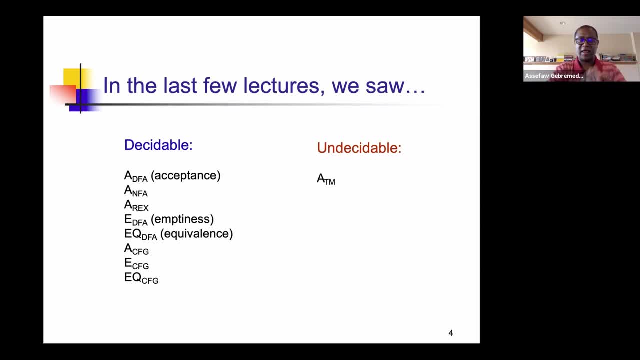 And we did something very similar when the underlying model now is not DFA, it's not NFA, it's not regular expressions but context-free grammars. And we saw those problems were all decidable On the undecidable one. the only one we saw so far was acceptance problem on a Turing machine. 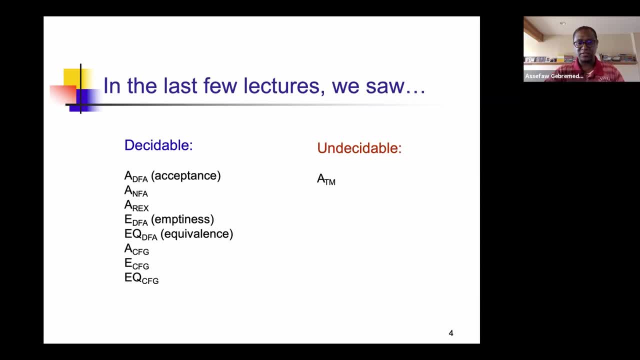 And the way we did show that was: we went through a process or a method called diagonalization. We looked into things that are both countable and uncountable and things like that, And so we established that this is an undecidable. There is no Turing machine that would decide this language. 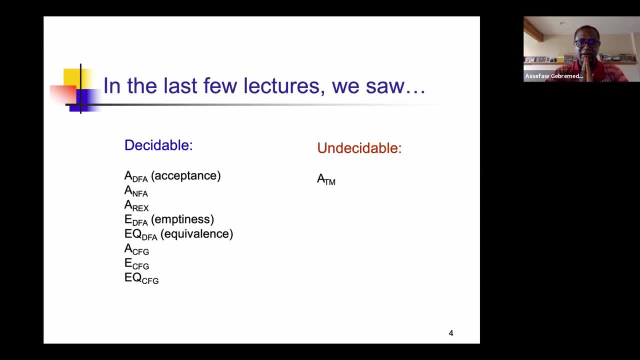 So if you look at this and you see now the universe and you try to divide it between decidable and undecidable, there are problems now, as we have seen. that would be of this kind: the things on the left and there will be problems of the thing on the right. 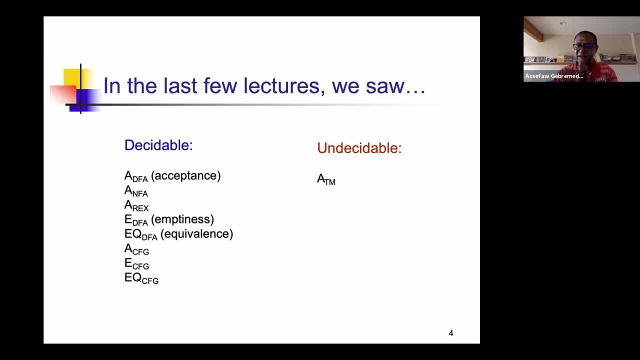 The fact that we have only seen one on problems that are undecidable does not reflect The universe. I am sure if we were to keep ourselves busy for the rest of our lives and try to see all the problems- language, wise, computational- 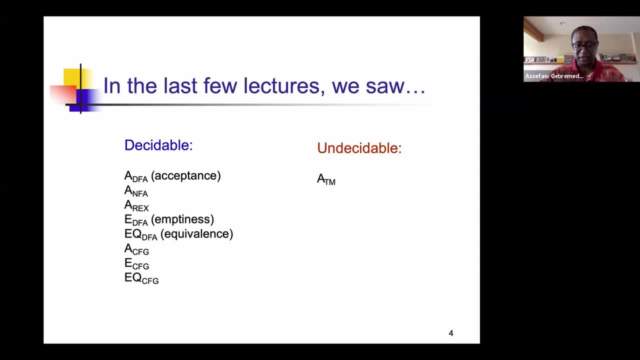 you know language wise membership problems if we were to give them names and start to look at them. there is a good chance that the things that are decidable are more in number than undecidable, but it's not as if there is only one here. 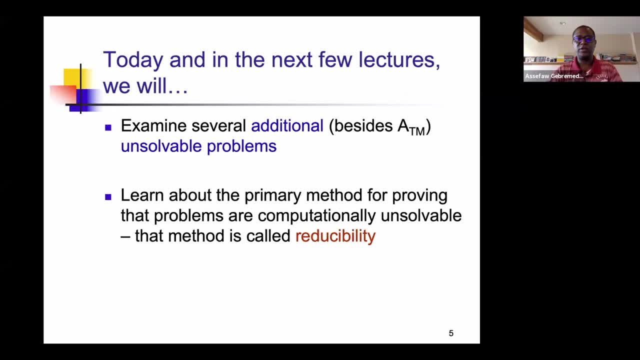 And so what we are going to be doing in this lecture and in the remaining lectures this week is going to find some company to this problem on language called ATM. It was a lonely one just by itself on that list, And so we're going to add more And the thing we do to get things more there. 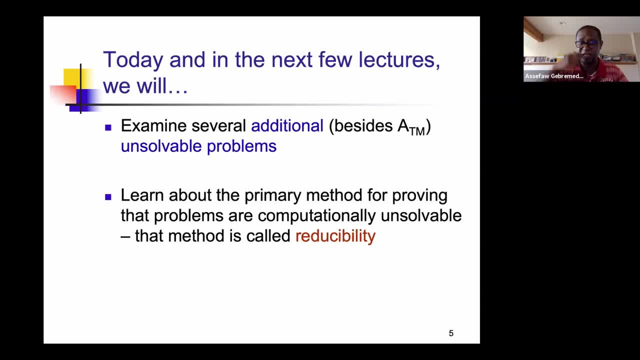 fortunately for us, is not going to be doing all the time like the diagonalization method and have gone through all of those steps to show that the new or whatever it is that we want to show now is undecidable. No, we have a better way to do it, And that better way is the subject of this discussion For today. 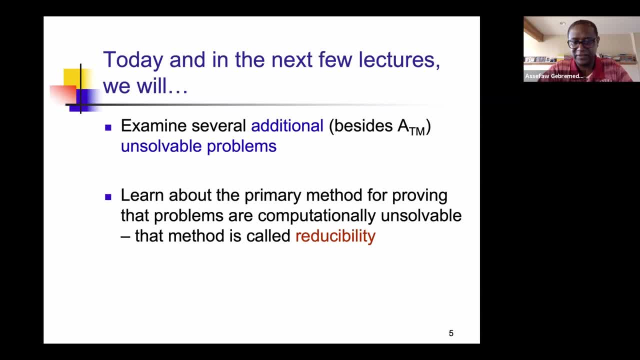 and for the rest of the lecture. thank you very much For the rest of the week and it is called reducibility, And that will be what we'll be talking about today and for what we will be doing the rest of this week. Reducibility is the title and now you have the reason for it. 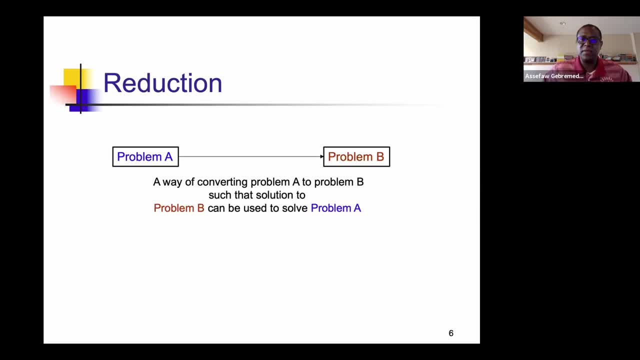 This idea of having to reduce one problem to another is not new. You've done this in many cases, and you probably haven't known it by that name, but you do it. So let me begin by having to give you a definition like this, and then I'm going to. 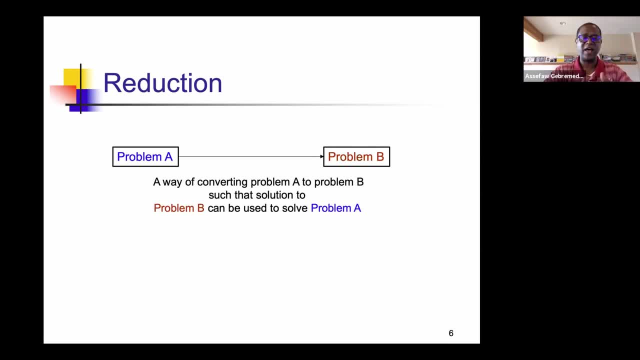 pause for a second and ask you questions, if you have anything like that Today. I didn't even ask you whether you have a question for me, I just jumped right into what we want to do, So let me remind you. anytime you have a question, of course you can unmute yourself and ask me, and I'll keep an eye on the chat area also- But the reduction, or reducibility, is what we will be using as our way to show problems that are undecidable when they exist, that is. 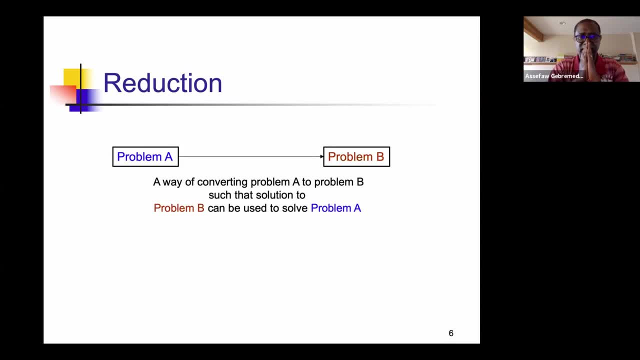 And so. but we want to kind of expand this one A little bit and talk about reduction in general. I've got problem A. I reduce it to problem B, a way of converting one problem to another problem such that a solution for the second problem can be used to solve the first problem is the idea behind reduction. 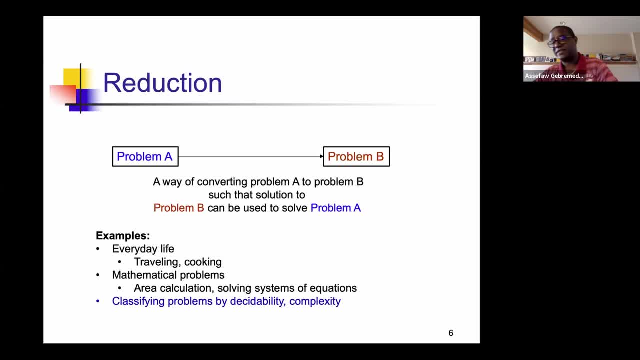 And we do this all the time in life. The book has got some very cool examples- something that you would enjoy- and I'm going to add a couple more, So let me give you some examples, So we'll begin by everyday life Examples of reducing one problem to another. As I said, we may not even call it like that. We may not even. 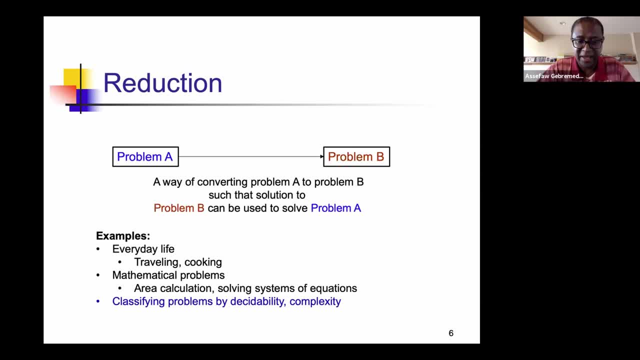 pay attention to it, but we do it all the time. In fact, if you pay attention to what we do, there's so many things that is automatic in what we do. that deserves some attention sometimes and a little bit of reflection, because it just happens and we don't realize it. but there is some technique, there is some way of doing it. So, for example, if you were- and this is an example that the book makes a reference to- if you were to travel, to a new place and it's a completely new place. you have never been there and you've done this couple of times in your life, I'm sure- and they're curious about where to go and what to do and things like that. 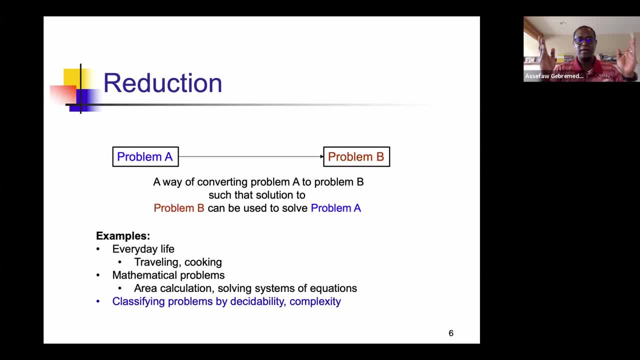 And so before you go there- if you are a good person and planned person, or maybe after you go there but you're staying in your hotel the first night- you would probably pick a good map or find Google or something, And so you've got a problem now that would make you look at the map and try to figure out where to go. 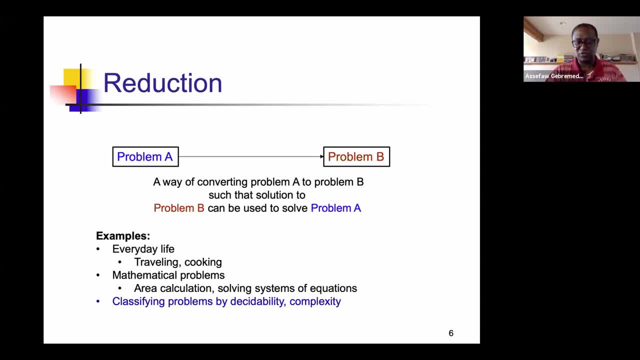 how to navigate, how best to use your time and so on. And so that question of traveling, exploration, that problem now has been reduced to a problem of gazing at a map and trying to figure out how things will be done. We didn't call it that. We've reduced that problem now to a problem of, you know, looking at things in a map Or consider one of the things that you probably would enjoy doing. 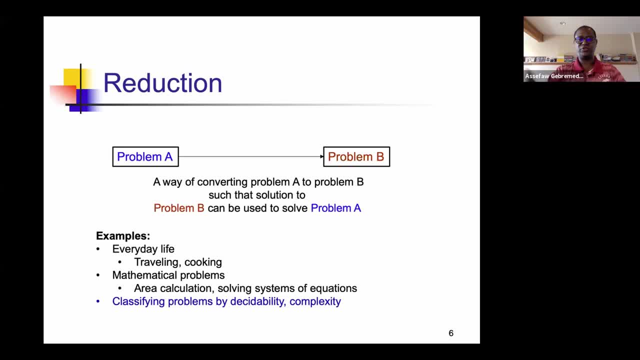 and that might be cooking, And so the idea of having a delicious meal that you would like to have now could be reduced to maybe looking up recipes, And if you're like me, you want to kind of change your recipe and ignore it and add your own thing. But there is some problem that has been, you know a thing that could be defined as cook, this thing. 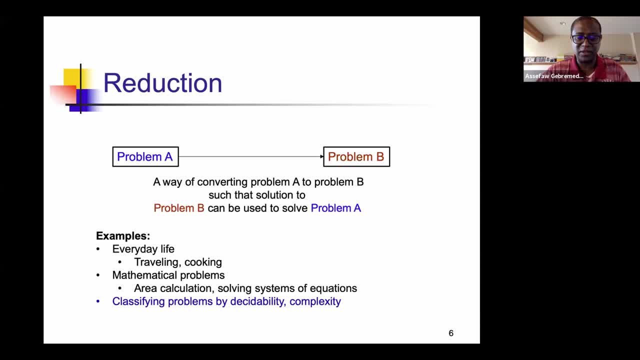 something nice, and then you've tried to reduce it to a problem, thinking about recipes, And you can even further go from that recipe and then it can bring it down to a problem where you would say: you know, go to the kitchen and get the knife, and get the chopping board. 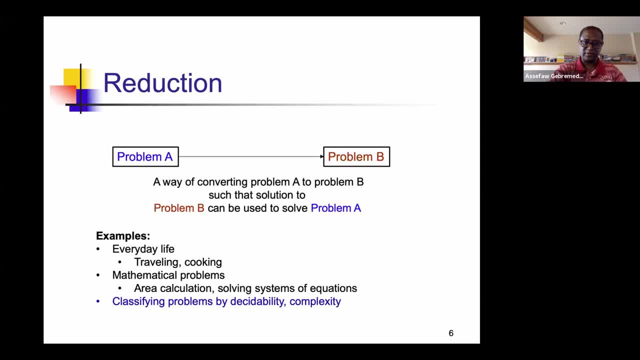 And do this, and then you know stir for a while and you know turn on the oven, And so you have turned the problem that was originally given into something else for the purpose of solving the original problem. So everyday life I could. I'm sure you can come up with much, much better examples than what I've just given you, But there is a lot of. 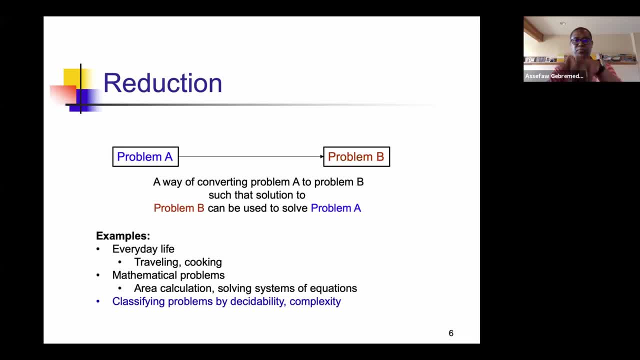 times when we would reduce one problem, we convert one problem to another problem, such that the solution for the second problem would be used to solve the first problem. And this could mean we can go further, and further, and further. So I could have A, B, C, but for an abstract way of representing it's enough for us to say two, So we can, we can always, you know, expand this problem. We could have its own reductions to other things. That doesn't change what we wanted to do. 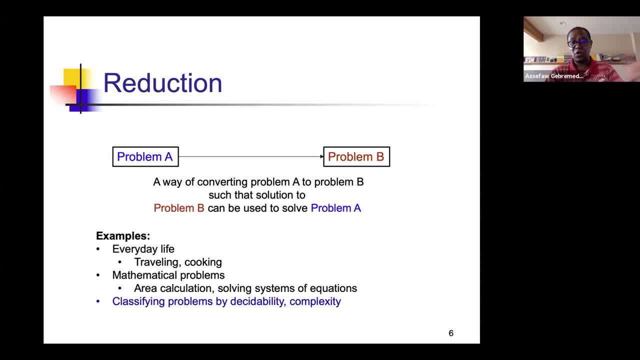 This is about everyday life, And this is enough of an example. But we can go to mathematical problems and see plenty, plenty, plenty of examples where doing something can be reduced to another one. For example, if somebody was going to tell you how, then we. 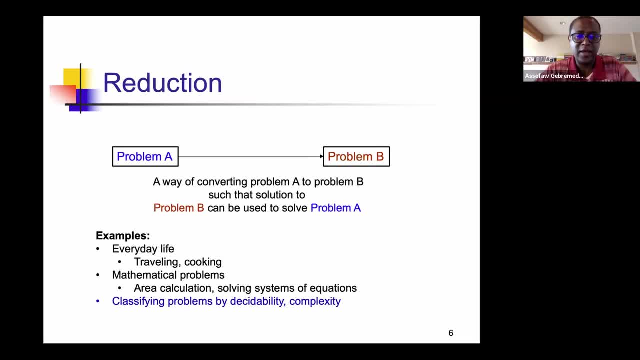 how to irrigate their- you know- plot of land now in one of these rural areas and you, they're all rectangular in shape and you wanted to calculate the area. you could, of course, go there, canvas with them and and find out how it is, and so on. But you can mathematically reduce this problem. It's an area, it's a rectangular. tell me the lengths and the widths and I'll tell you the area. So if you reduce the problem of area calculation- this is not a big example, but it is at least mathematical area calculation- into when it is. 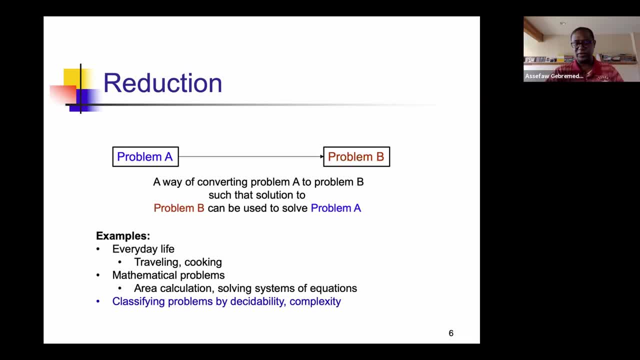 a rectangle, to finding the lengths and the widths, or if it is another shape. if it's a circle, then you've got the area calculation reduced to finding the radius and that's that's all you really need to solve that problem of calculating the area. 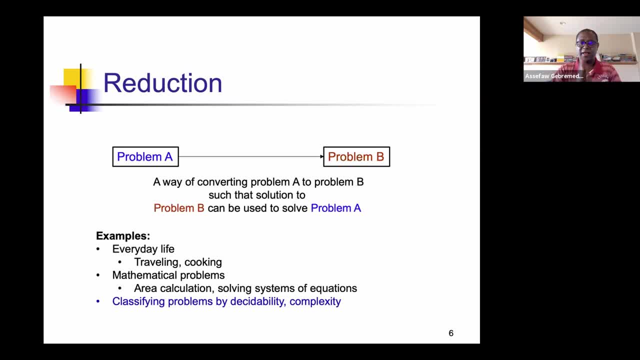 Or you can consider solving systems of linear equations, and I have mentioned this one and maybe you will notice that every now and then I, whenever I get a chance, I'll try to remind you, and some of you might not have appreciated those kinds of good courses. 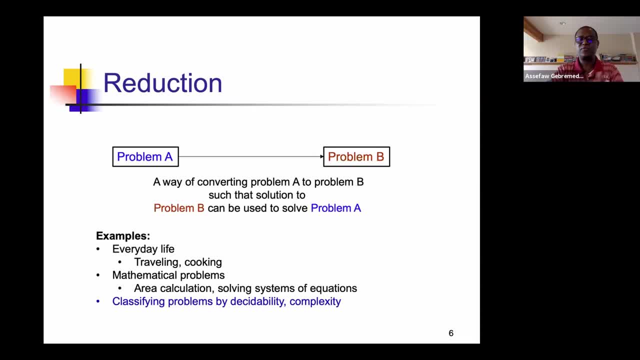 To the extent needed. but you've got a system of equations to solve. Now you know what to do. So AX equals to B. Sipser, the book tells you that you're going to infer the matrix A to get solution for X. 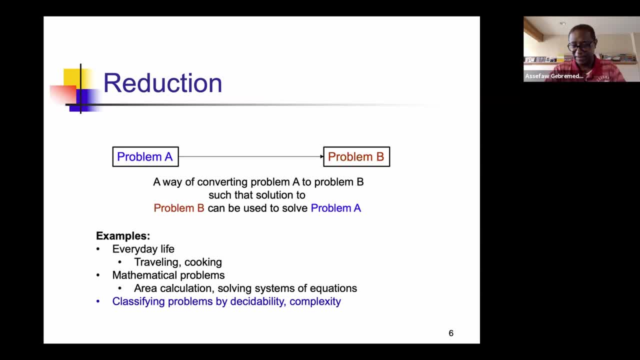 So X will be equal to A inverse B. That's what it would be mathematically. That's correct, but you will not do that. computationally. That's not a good idea. You would instead turn the matrix A into decompose it into its lower and upper triangular forms. 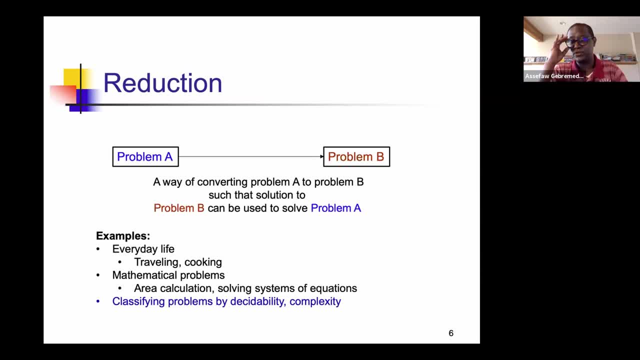 And if you remember when we talked about Turing machines And then we were talking about algorithms, how they came about and so on, We saw all kinds of examples there, But one of them was the Gaussian method, Hundreds and hundreds of years old method That is what you would do. So you've reduced the problem of solving a system of linear equations into factoring a matrix into L and O, inverting the matrix. Mathematically. they are equivalent and they are doing the same thing. 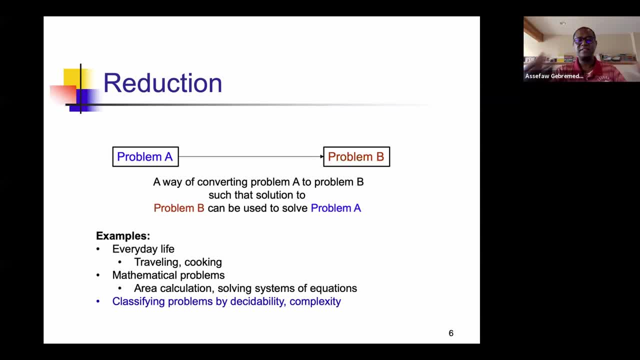 But computationally. I warn you you don't want to do that, But but this is, this is what you would do, So don't do it. mathematically, Our subject is the third one We are now going to be. is this reduction to do things around decidability? 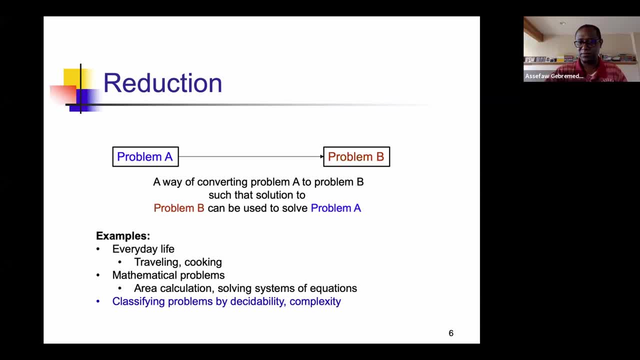 And the very same idea of having to reduce one problem to another for having to classify problems is also used not just for decidability but for complexity. This book has got this three parts. I've told you many times, And our course is largely focused on the first two parts. 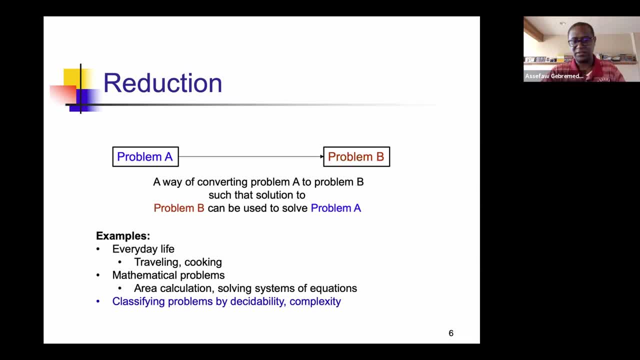 And, happily, are about to finish this second part about computability. we are in chapter five now, and and so by the end of this week we'll kind of make our way through it. but there is a third part that is a huge chunk in the course. that's about complexity. we'll just have a bit of it in the last. 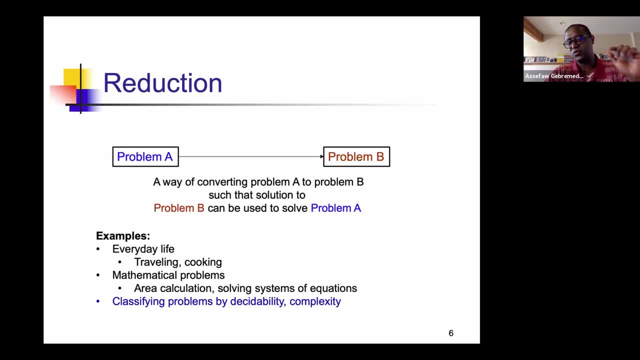 week. just an introduction, but there too there is a way to talk about one problem being reduced, another one to show that one of these problems was intractable, it was difficult- and i show this other one is also like that- to classify it by having to reduce. so for our purposes we are going. 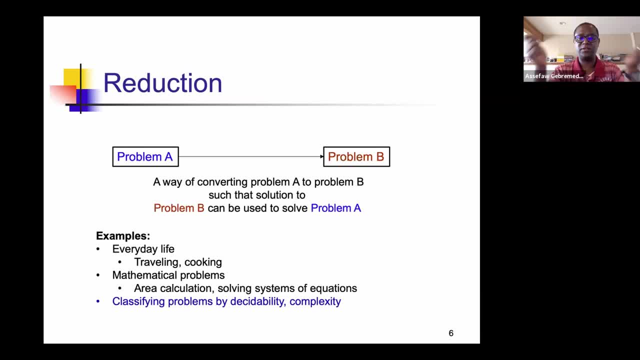 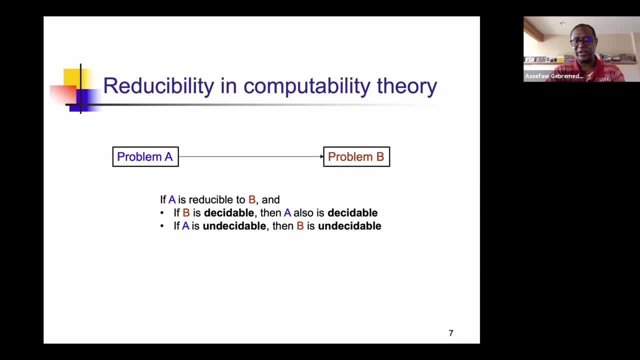 to be using now reduction, reducibility to show that a problem is decidable, to classify it as indecidable or undecidable. this picture, you need to have it and i wanted to plant it in your head so that you would remember it and you can tell your friends and it will become so very natural. 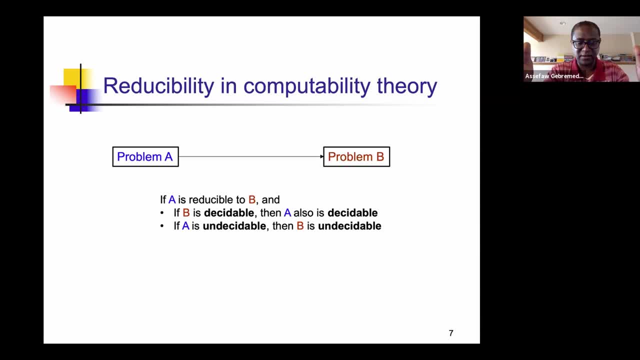 to you. you will be surprised. some people sometimes get it confused. so so your goal is now to show reduce, to use reducibility, to show that the problem in our case, for the rest of the discussion here, actually is to show that a problem is undecidable. so we have established, and i'll 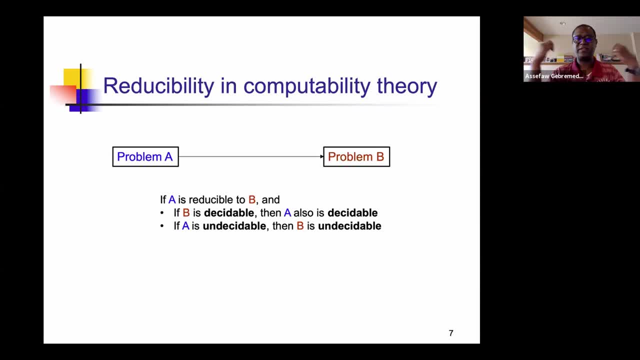 tell you the place where people make mistakes. we have established that this idea of having to reduce. reduction is about having to convert problem a to problem b so that the solution for problem b could be used for a problem to solve a problem for solution to find a solution for problem a. that is what reduction is. that's what the cooking was that. 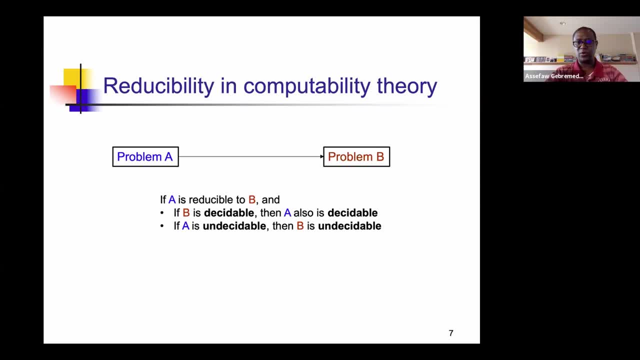 was what the troubling was. that was what the linear system of equations were. we were solving this piece to get the solution to the original one and therefore we reduced when b is decidable. so here is now: if a is reducible to b- and it doesn't necessarily mean so you can always reduce. 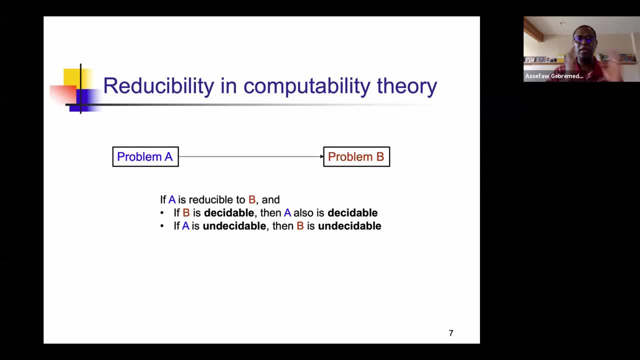 one problem to another. by the way, that's the art, that's what we will be learning now: reduce one problem to another. but if it is when, if a is reducible to b and if b is decidable to b, the new one is decidable, then i can go back and solve a. then i know than a also is decidable, why. 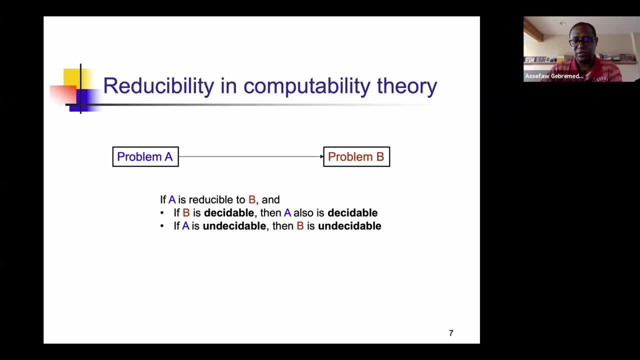 because i could use the solution that I found for b to go solve problem a. therefore, if a is reducible to b and if b is decidable, then a also is decidable. in the other case, if a is undecidable, then B is undecidable, and this is undecidable. 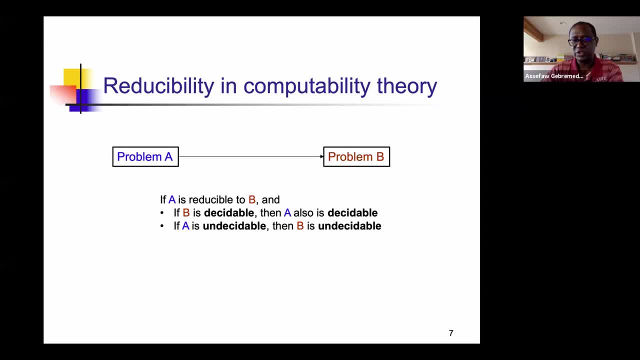 second part is where we would need it most. The first part is everyday wisdom. Computer scientists: now you know how to write code, you write program and sometimes you find out something that is something that you would need as a subroutine, something that could be used for a 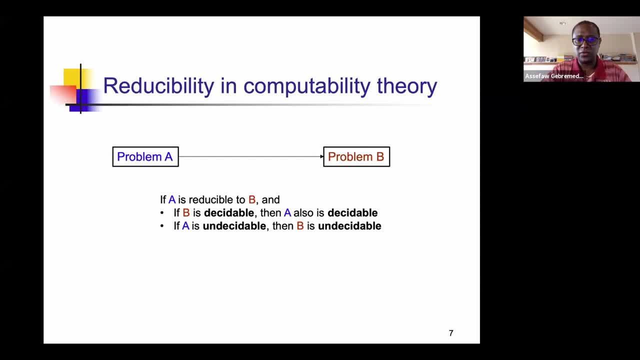 general purpose, And so you do that and then use it to solve your original problem. You do this all the time You would do. you don't even think about it. Sometimes you call it a good software engineering practice. Maybe you have an algorithm now, a piece of code that probably would benefit. 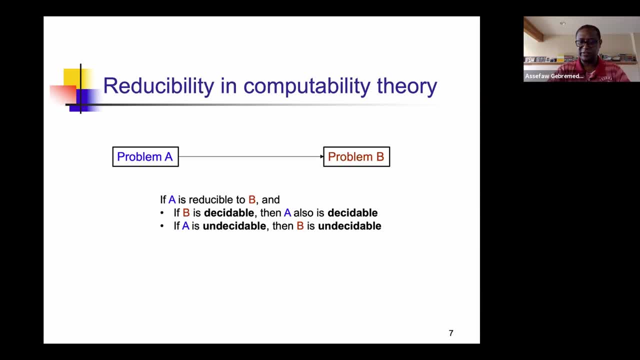 by having to chop it down into reasonable things, And we've got functions or subroutines, whatever you want to call them- A, B, C, And so you glue them together to solve the original problem. So you've got this idea: when you reduce problem A to reduce B, when B is decidable, the new one, 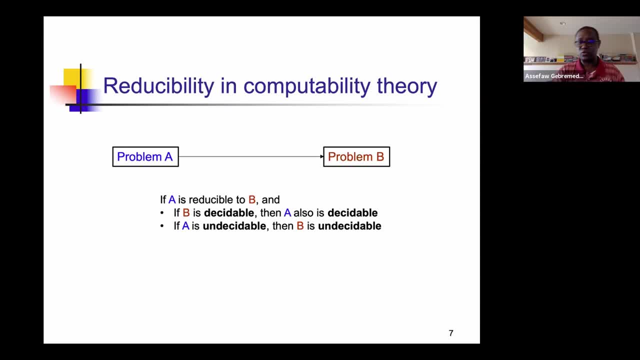 to use it to solve A. this is a usual practice and you automatically do it and it was always there. The second one is the one where I am wanting to tell you now a little carefully: You now have a different use of this same idea for having to show an impossibility result in a way. So if A was 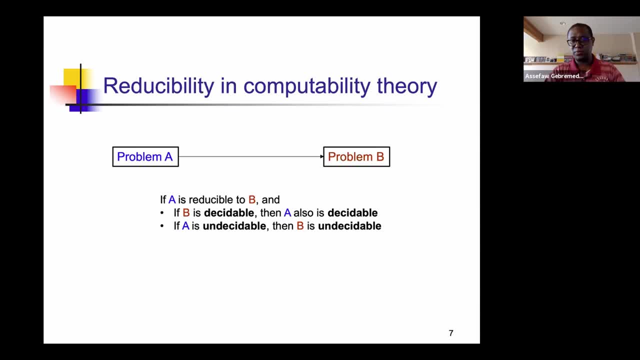 undecidable, then I reduce it to problem B and the reduction has happened. So if A is reducible to B and A is undecidable, then I can conclude that B is undecidable. So now I have a few. 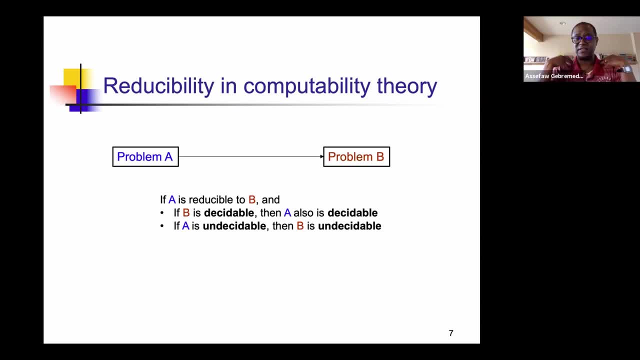 a new way to show a result. What I have done is, if I knew, and I know now, I know now. there is one problem at least I learned in this class, we've learned in this class. it's called ATM. it's undecidable. 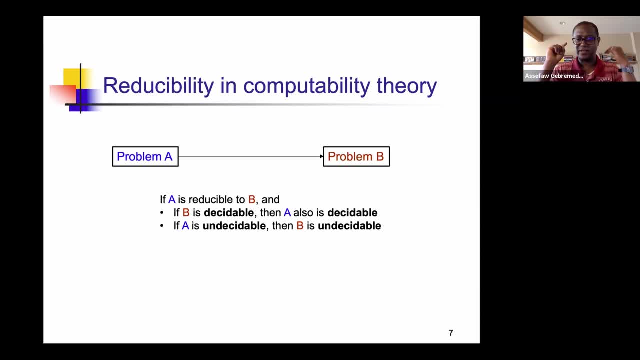 So if somebody comes and asks me a new problem whether it's undecidable, I'll tell them: oh, let me see if I can convert that ATM into your new problem. if I can successfully do that, because I know A is undecidable, then I can conclude that B is undecidable. And why is that? 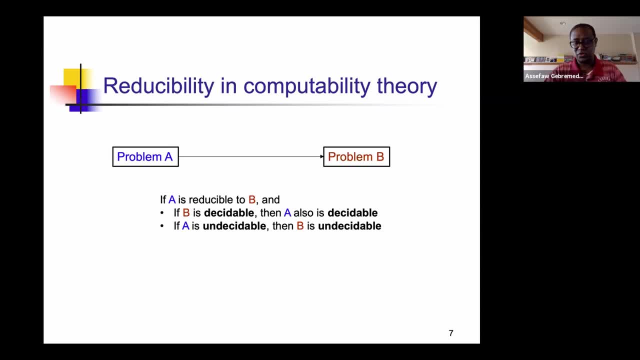 Because the first statement shows you that problem A cannot be any harder than problem B. If I can solve problem B, if it is decidable. if B is decidable, then A is also decidable. So that same argument tells me that A cannot be any harder than problem B. So if I know, 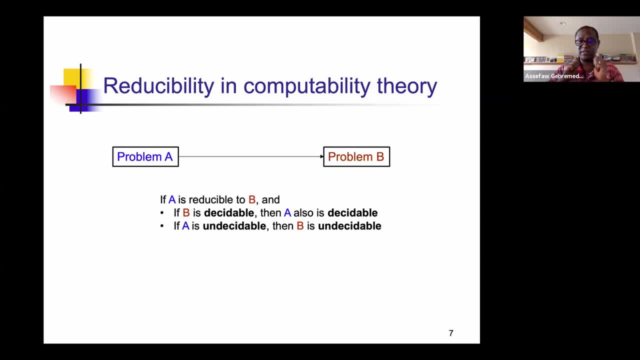 A is undecidable, then B also has to be undecidable. Otherwise, if B was decidable, then I could use the solution for B to go back and solve A, which would be a contradiction because I know undecidable. so therefore, this is now going to be our way of showing something is undecidable. 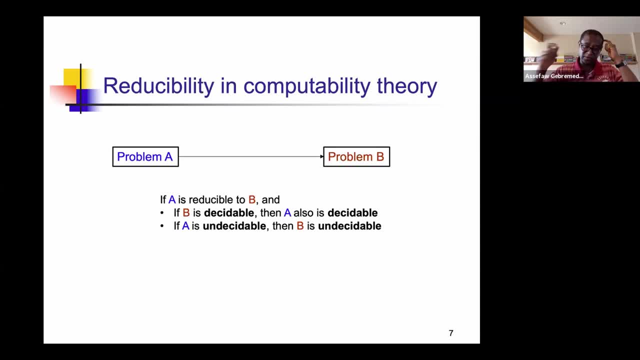 counter. when he had to do this uncountable stuff and so on, he did diagonalization method atm because we didn't know anything else. we had to do the hard way, we had to labor ourselves and get using the diagonalization method to show that undecidable. now that we've got at least one, 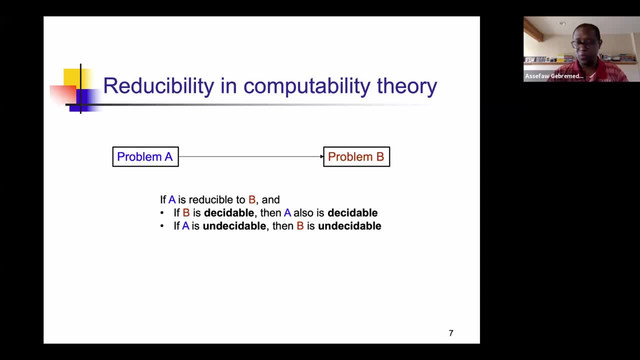 problem. we're going to be acting like lawyers, we're going to invoke this thing. okay, now i have this theorem, this stated in the law, in chapter this article, this and this, and therefore i'm going to apply to this case and therefore this case is, like this, guilty or something you argue. 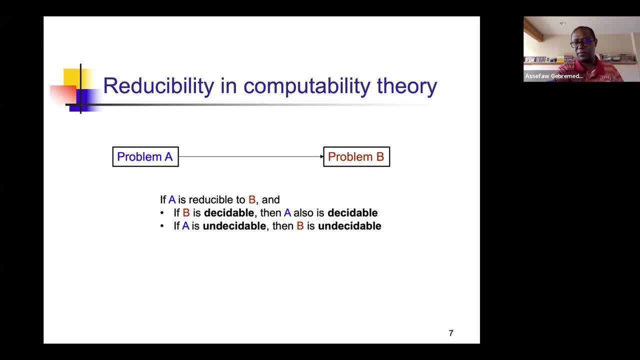 for it. it's much like that, so we're going to now take the problem and reduce it to the new problem. the place where i want you to be careful is where people misunderstand how the reduction would go. if you wanted to show a problem is undecidable, you start with a problem. that is. 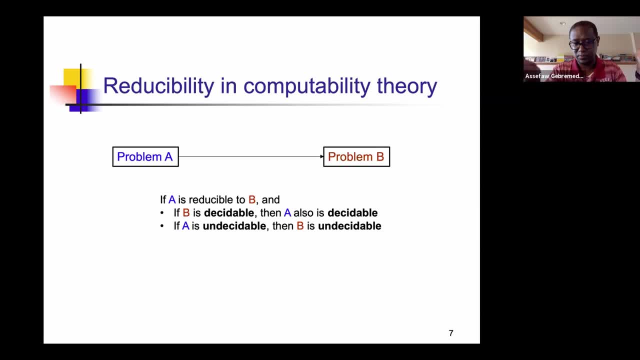 non-decidable to be undecidable and you reduce it to your problem. when you have done that successfully, then you can argue that the new problem is undecidable. that is what we'll be doing, and we'll see a number of examples, and so, before i get started, here's an example and we'll stare. 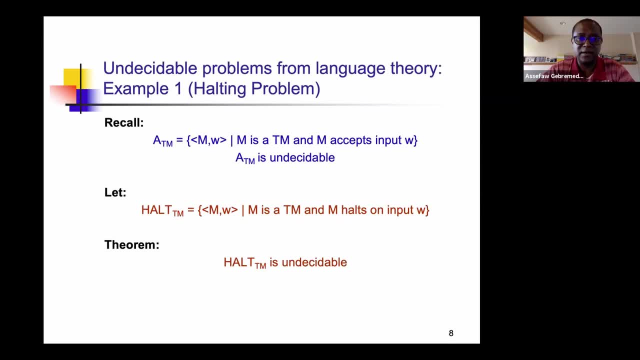 at it for a second, but let me see if there is a question you have so far from what we are discussing so far anybody else got any questions? just so i know that you're following me. no questions, it's fine. it's difficult to tell me when there are no questions, so i'm going to 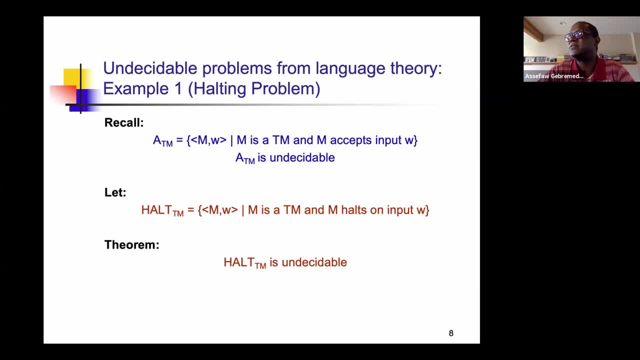 ask you few questions, but, um, i'll just interpret silence to mean no questions. all right, uh, okay, so. so make sure to to to always unmute yourself and ask, okay, so so now we are going to be doing. i know we know what, we know what we are after, we know the right way, the right direction to reduce. 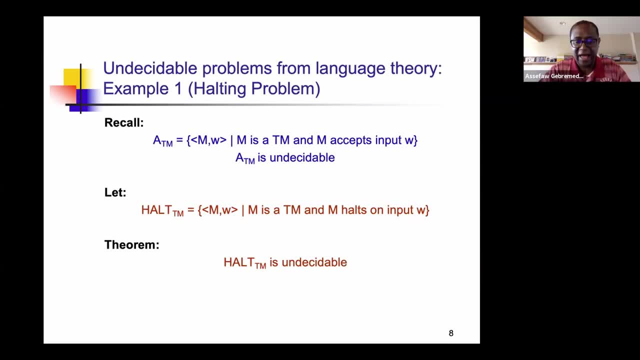 problems and we know how we are going to, generally speaking, apply reducibility to show undecidable problems. that's what we are after. i know what we are after, if you knew it mentioned. so now, what are you going to do after? what are you going to do after? this whole thing will get better. let's say, for example: you say what i mean. if you only want something that theそれは профессion себя need to reduce so we can reduce majority of this opportunity, we are just going to be discarding the value. to get what? yes, the idea that this idea is that problem is undecidable every time we h debra Mussaefi. 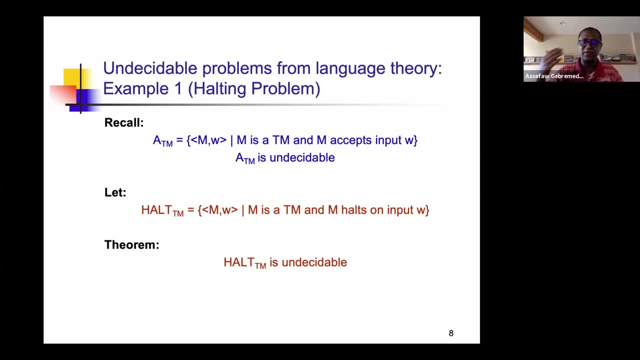 we are up to, And I'm going to show examples, Just like we have faithfully gone through things and we have seen. we'll say four examples, five examples, six examples, four decidable problems. we will do today four examples And so. 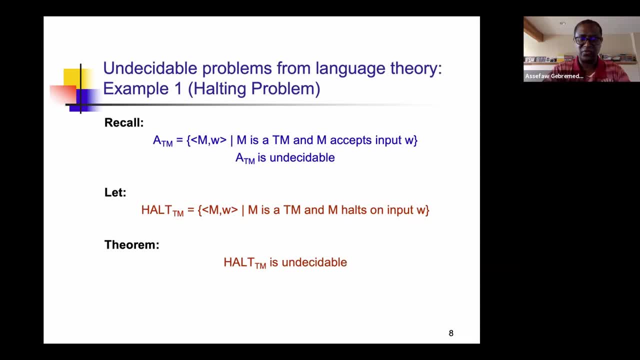 we'll count, and if we not have enough time and we don't finish all four of them, there is nothing to worry about. We pick up where we stopped last. next time We continue this discussion, But that's why they are numbered, And so we'll see. 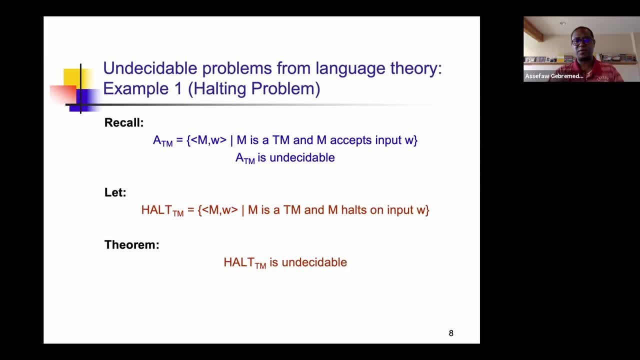 the first problem. And the first problem is the most famous problem. It's called the halting problem. Some of you might have encountered it, Somebody might have told you, or you might have encountered it when you read something. It is called the halting problem and it has to do with steering machines, Because we need 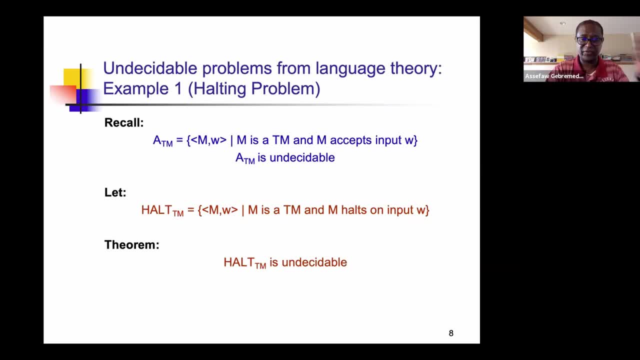 this ATM quite a bit. it's going to be our friend for a good chunk of the time we have today, Because we're going to use it to reduce. We're going to reduce ATM to this problem and therefore this problem is undecidable. That will be the 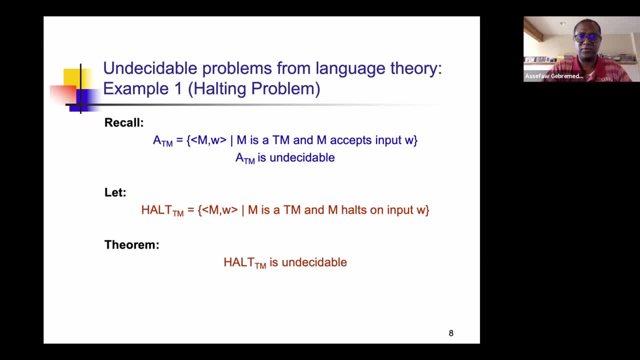 the narrative. That will be how the story will unfold today. Four Many of the examples, except for the very last one, and you will see why. So, therefore, I'm going to just remind us what ATM was. ATM says we're given a Turing machine, M, and it accepts input. W is the language, and so we know that this. 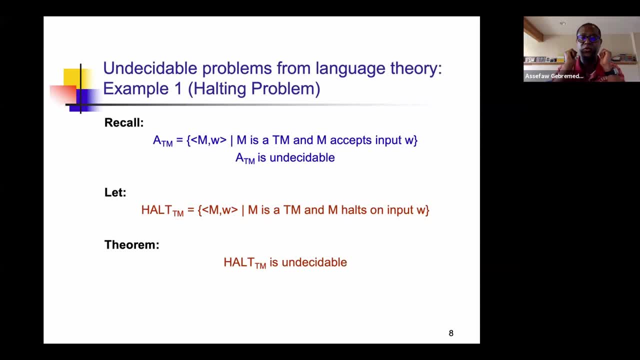 is undecidable, And so we're now going to look at the problem called halting. And so we've got Turing machine M and we are going to decide: or the language says M halts on input W. The reason ATM is undecidable is because it would accept and it could either. 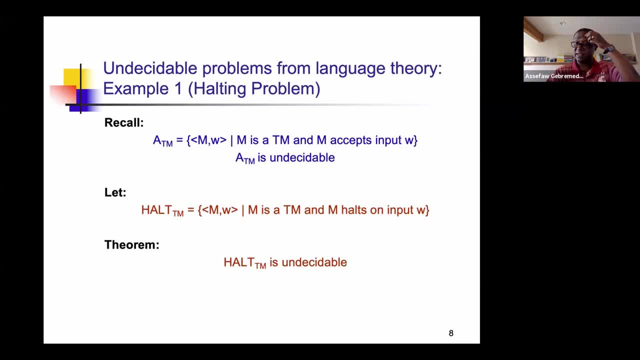 reject, or it could run forever. And it's because we can't tell apart those two. That's why it was basically undecidable. So this halting problem now is a tweak on that one, in some words. So if we have a Turing machine, can we know? 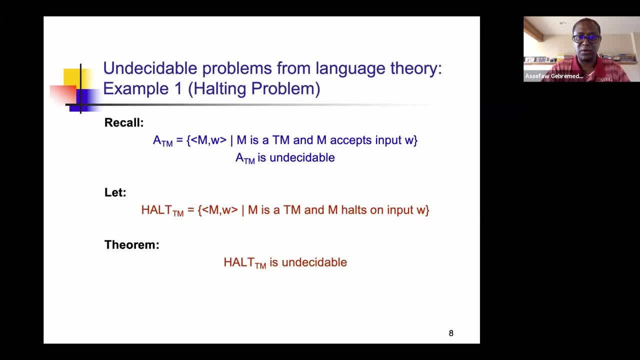 whether it's goal to halt or not, And that problem is called the halting problem And the result we have. just like we've been doing so far in the past lectures, I'm going to follow this format. What I'll tell you, the problem I'm going to. 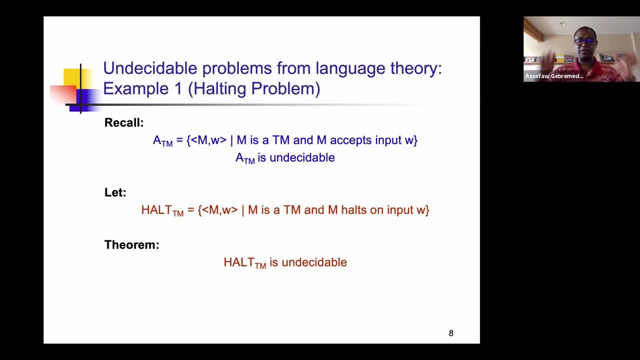 follow the language, Define it, tell you the result, and then we'll spend a couple slides proving it. So the result here is HALT TM is undecidable, And this is going to take us now through a proof technique that is going to be familiar. 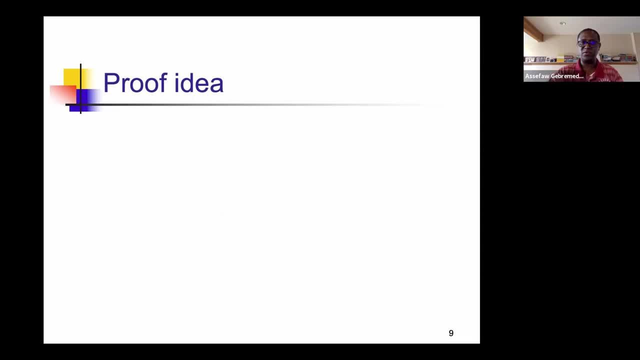 So we are going to be- or rather the same pattern, We're going to be- using it for all examples that we will be doing. Sipser has got this good idea kind of style where you know proof is broken into first the idea part and then 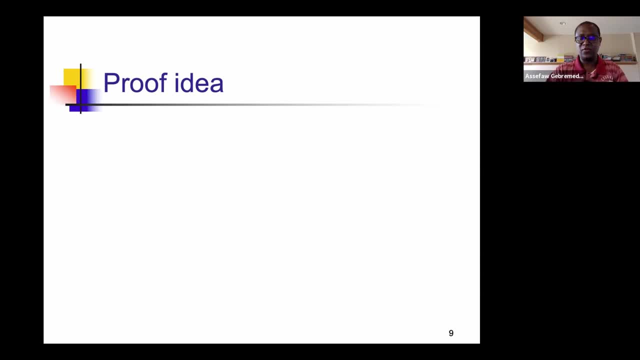 the actual formal proof part. I'm going to use that especially for these ones because it is particularly useful, And so I'll start with the idea, talk through it, and then we'll have the formal way in which the you know the machines that are. 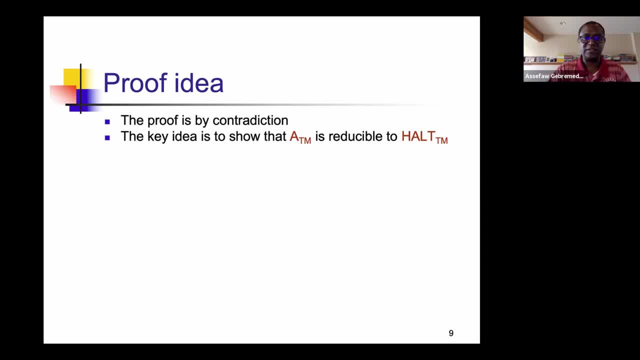 needed to complete the proof are formally presented. Okay, Whenever we have to show another problem, one problem is- I shouldn't say another problem, one problem is undecidable- is to reduce undecidable problem to it and then show that, because the problem that we have 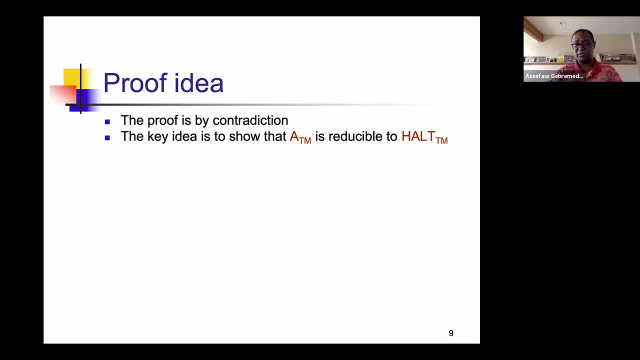 reduced it from is undecidable, then this one is going to result into a contradiction. So this is going to be all proof by contradiction. That is one keyword. So the key idea, then, is to show ATM a problem that we know is. 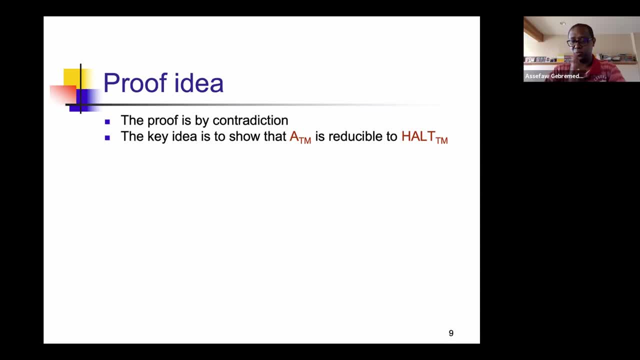 undecidable is reducible to this problem. So if this new problem, now HALT TM, were undecidable, then we can go back and argue that ATM would have been decidable. but we know that ATM is not decidable and therefore, 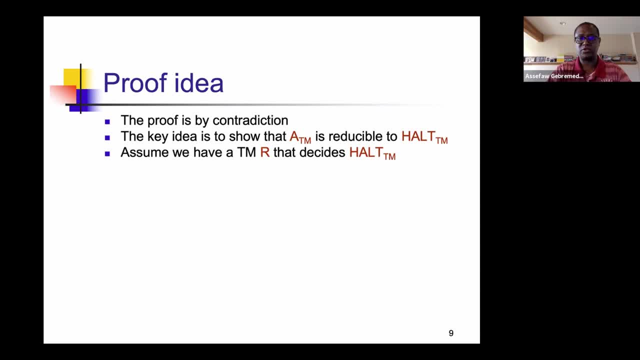 HALT TM cannot be decidable. That's the idea. That's where the contradiction would come, And so every place now. so this is the common ingredient for all of the proofs that we will see today. In doing this, there's another common thing that we 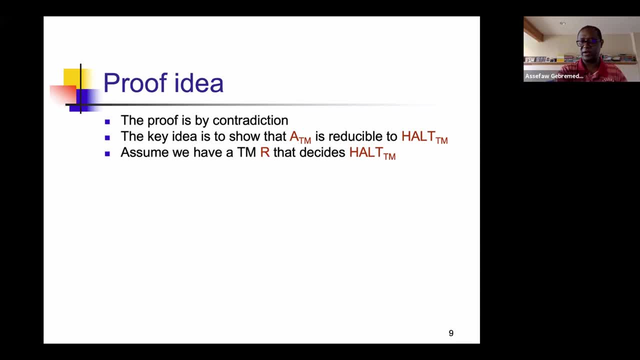 would we will have. for the purpose of arriving at the contradiction, we will assume that there is a Turing machine that does that reduction to reduce it, And for that reason we'll call it R. So every time you see me now I'll call that Turing machine, R. So assume that we have a Turing. 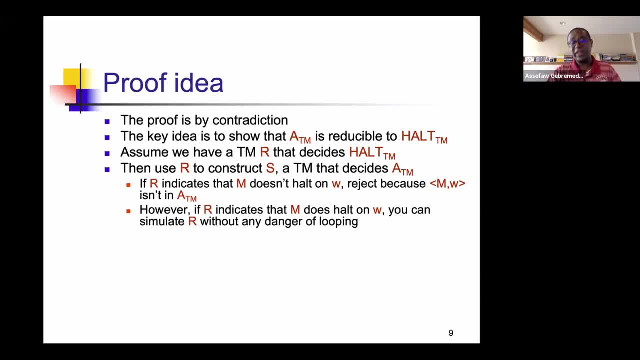 machine R that decides HALT TM, Then what we could have done is run this machine and simulate it to see whether what we can do for a Turing machine for our original problem for ATM- But we know that that is the Turing machine that we would do to this one may run forever, So that simulation is not going to be a 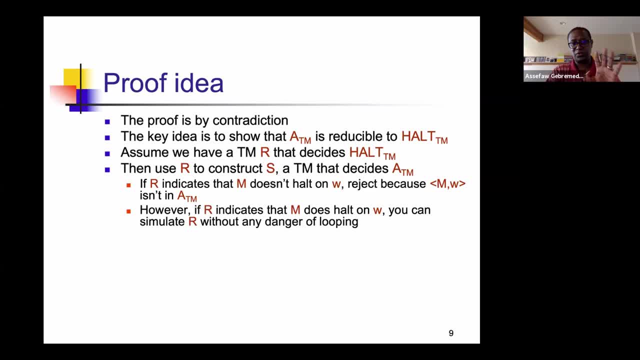 good idea, And so, therefore, instead, what we're going to be doing is going to be the following: So we're going to use this assumed Turing machine that we have called R to construct a Turing machine. that's S, that's our simulator, So you will hear me. 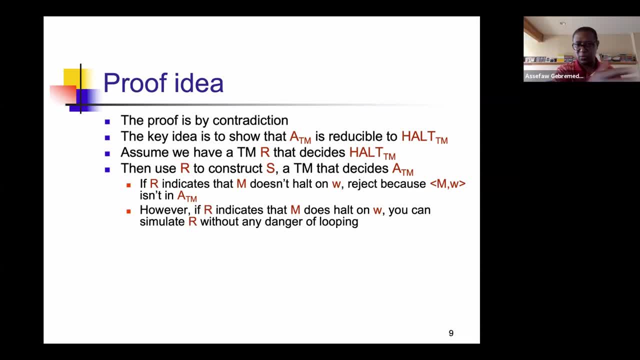 use these names, R and S. The R is for the one that's reducing and the S is for, roughly speaking, the one that's going to simulate. It's going to use this one to come up with what would have been done for the original problem, the original. 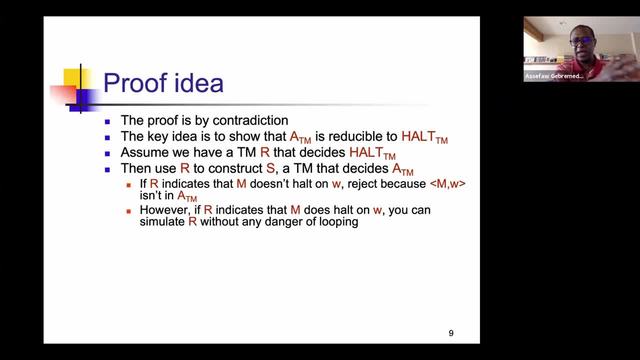 undecidable problem, in this case HALT 2M ATM I mean. So we're going to use this one to construct a Turing machine that decides ATM? How are we going to go about it If R the one that we have used now, assumed? 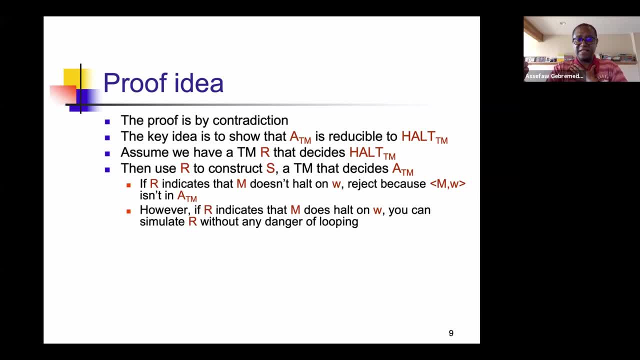 is going to decide. HALT 2M indicates that M does. M is now the input. by the way, M is the Turing machine that we had in the beginning right And W is the string that it is working with. If R indicates that M doesn't HALT on W, we reject because this M- W encoding is 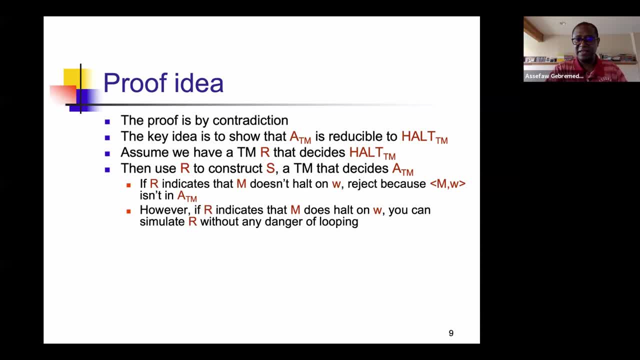 is not a member of ATM. However, if R indicates that M does hold on W, now we can simulate R without fearing that it will loop forever, because we have at least avoided that one, because of the assumption that we have made. Therefore, if the Turing machine 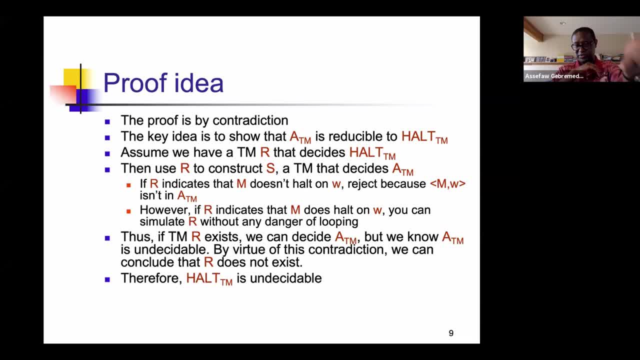 that we have assumed now actually exists. it means that with these two steps that I showed you, now we can decide the original problem, ATM. but we know that the ATM is undecidable and therefore we have arrived at the contradiction. Therefore, hold to M is undecidable. 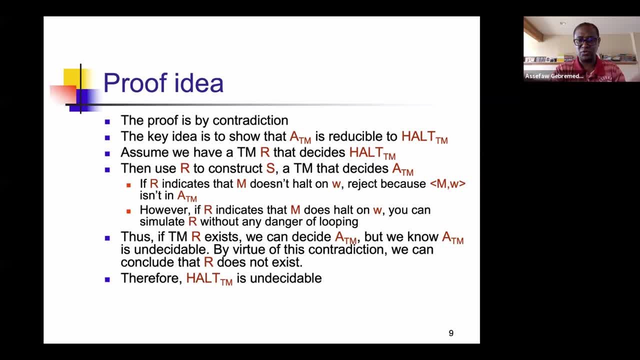 So, if you have paid attention to the argument I have just used, hold to M and ATM are very close to one another And the only decision that we have made with hold to M was we just wanted to determine whether the machine was going to hold or not. 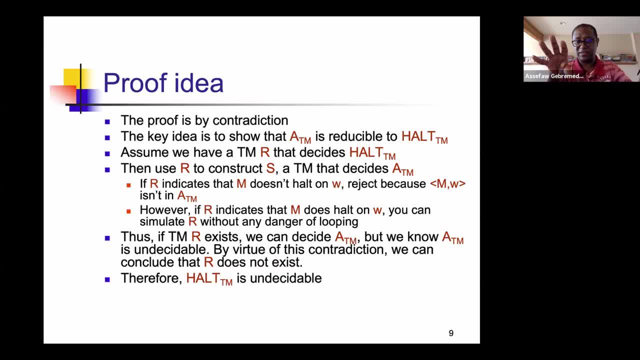 But that's essentially what the idea was: for ATM to be undecidable in the first place And therefore, if these were decidable, we would have arrived at ATM being a decidable one, and therefore that cannot happen. That's what this proof idea is. 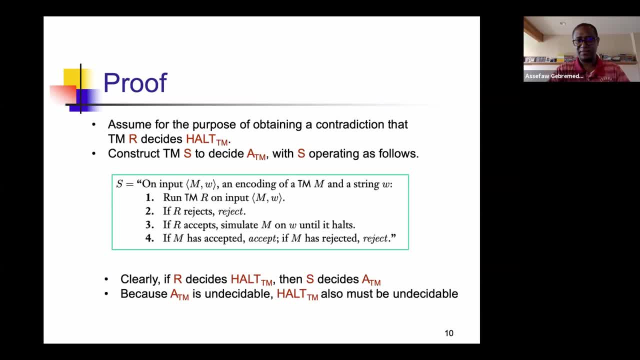 So now that I have money to get this one onto one slide, let me show you how the formal proof would be written. This is going to be very much like a duplicate of what I just said in the previous slide, except that it is formally stated. 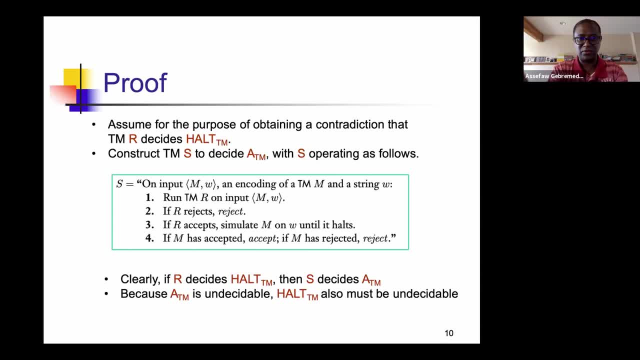 But I want you to know how it's formally stated, partly because you would be doing this in your homeworks, but also because this is the way you would present it if you were to be asking someone else to, not just in your homeworks. 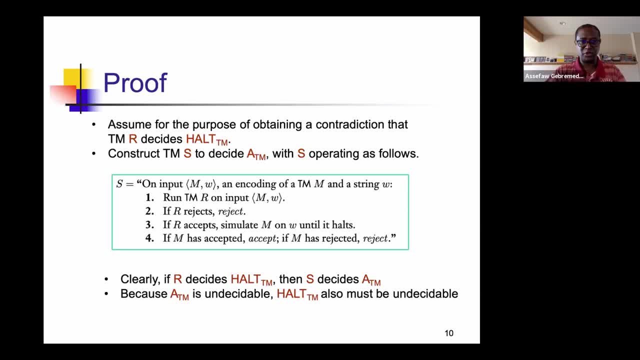 So assume, for the purpose of obtaining a contradiction, that we have a Turing machine R that decides our new problem. hold to M. We're going to construct a Turing machine S to decide ATM, with S having this operating in this fashion. So now is the description of S, the high-level description. 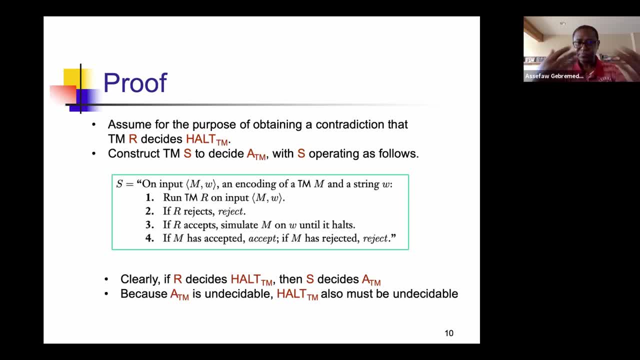 of S, as we like to call it, on the input, the machine M and the string W, The encoding of that one together, And it's an encoding of the Turing machine and the string, And so we run the Turing machine R that we assumed on this input. 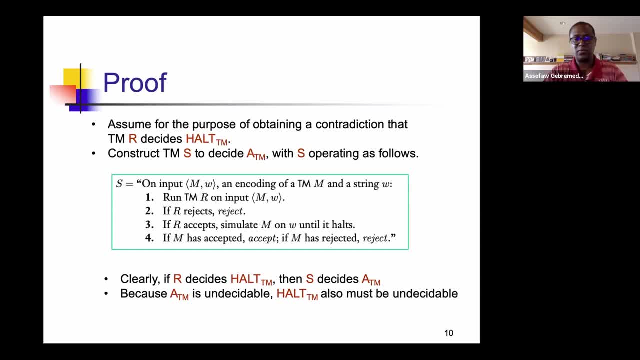 If R rejects, we reject. R is the one that's going to decide the new problem, the hold to M. If R accepts, we simulate now. If R accepts, now we know the simulation is not going to run forever, And so we simulate M on W until it holds. 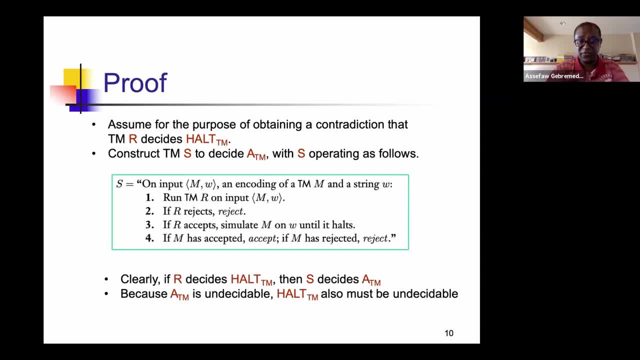 If M has accepted, we accept. If M has rejected, we reject. If we were to be successful with this, then we have just shown that ATM is decidable, But we know ATM is not decidable And therefore we have completed the proof by contradiction. 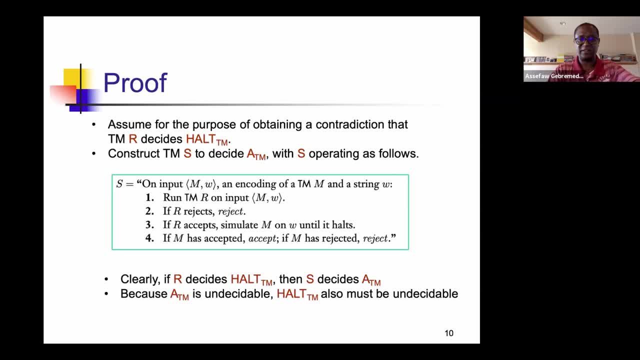 So, as I said, this is just a restatement of what I showed in the previous slide, except that I have the green box showing us the formal way to state what the Turing machine S would be in the presence of the assumption that there is this Turing machine. 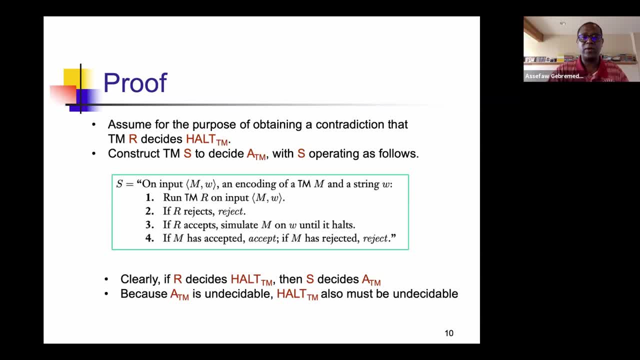 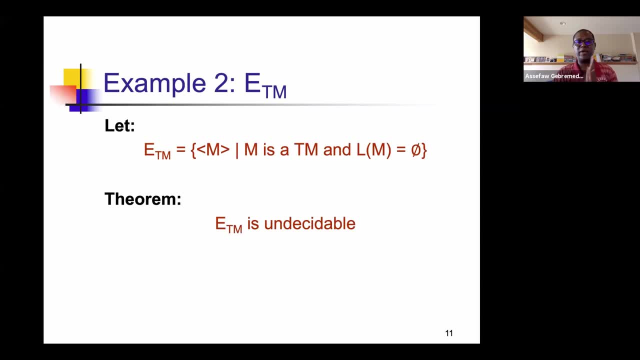 R, that would decide hold to M. Therefore, we added one company. So keep counting. ATM is not alone anymore. Hold to M is added to it. So let's come to example number two, And this time we're going to work with the kind of guys. 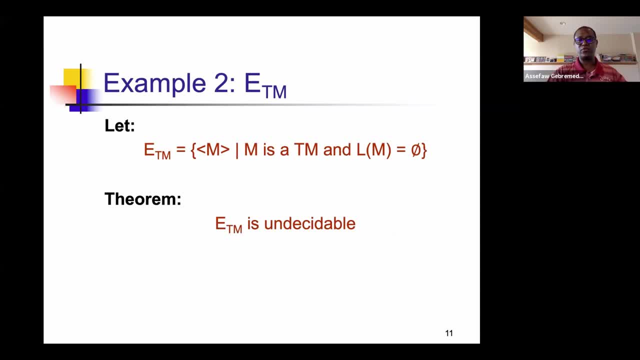 we call EEE in the decidable world And those were. when the language is empty, the E there is for empty. So we have ATM. the language that says M is a Turing machine and the language of the machine is empty say. 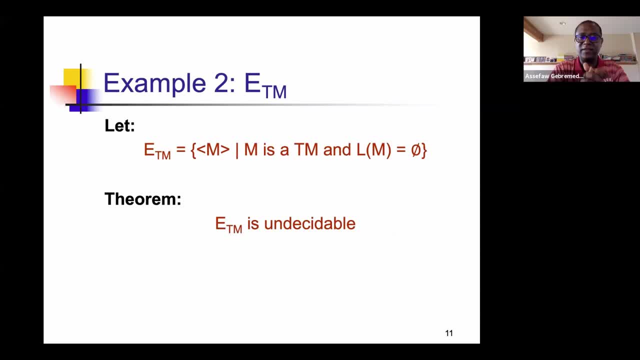 And we're going to assume that it is decidable, And the result is another company for ATM And this one is also undecidable. The proof, very similar idea to what we did before. We are going to assume that ATM, our now subject. 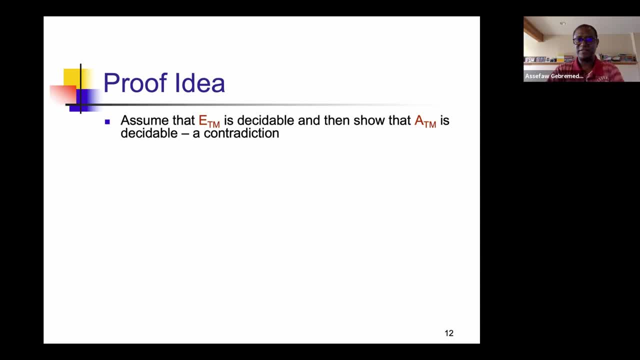 what we're going to investigate: is it decidable or not? We are going to assume that it is decidable and then show that it is decidable by contradiction. That means we are going to reduce ATM to this problem, And then that's where the thing will happen. 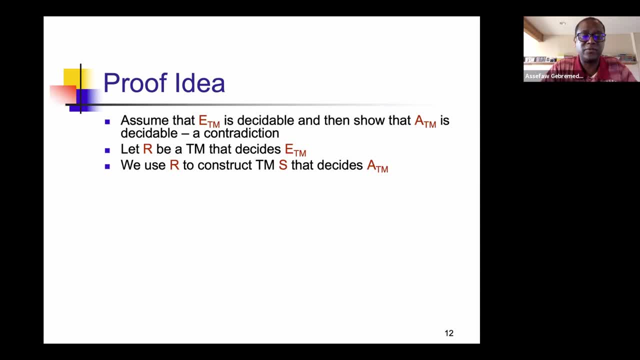 A contradiction will happen. And that reduction, that reducing with the Turing machine, we'll call it R, just like we did before. Let R be the Turing machine that decides ATM, And we are going to use R to construct a Turing machine S. 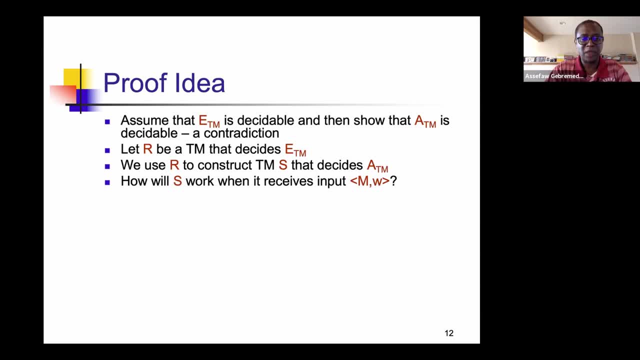 that decides ATM, only to arrive at a contradiction. But how is S going to work when it receives this input? Remember, this language now is the empty language, And how is it going to do So? I'm going to give you one idea. 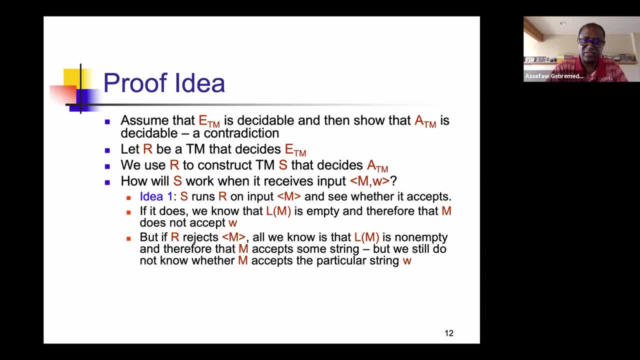 And this is similar to what we have seen, I think, a few weeks ago, wherever we had, I think, a few examples, not a few weeks ago, a few lectures back when we had one idea and we say that it doesn't hold water. 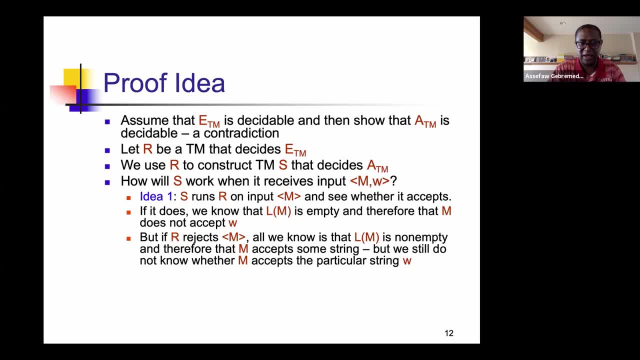 So it kind of takes us to a place where we can't argue any further with it, And so we give up on it and then pick up another idea, just to see- And that's how- our first thought might not have worked. So I don't want to get to the right idea right away. 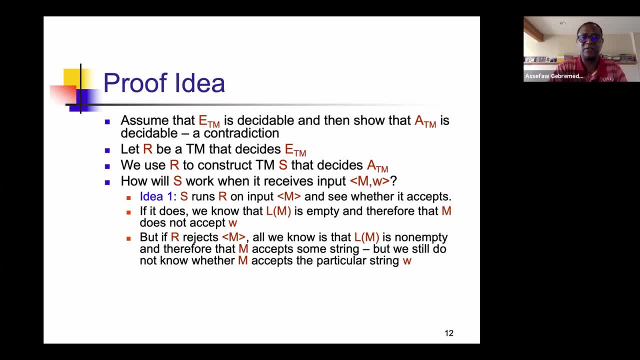 So let's first work with an idea that might first come to mind. So that will be. we will run S. the one that is going to decide ATM is going to run R. the one that is deciding ATM on this input, the encoding of the machine. 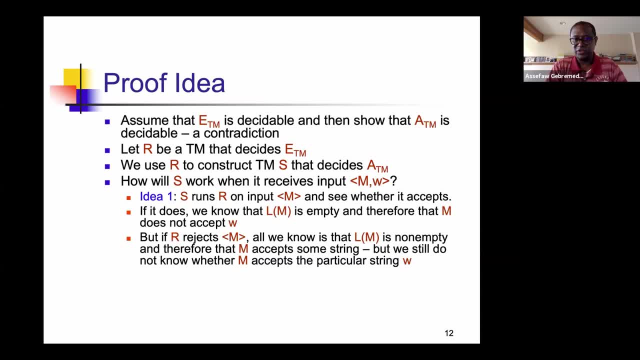 and see whether it accepts. So the machine now, whether it accepts R. when it accepts R, remember what it is doing. This is about the empty language. If it does, we know that LM is empty. That's why it accepted it. 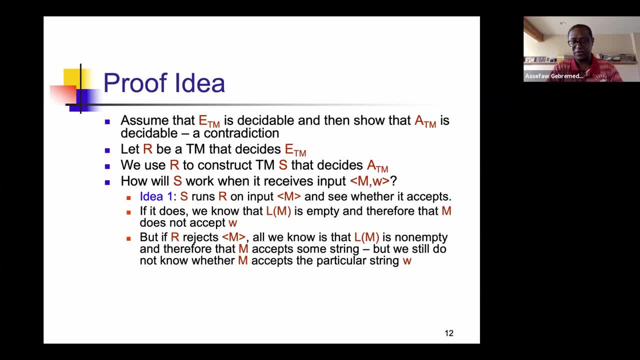 And therefore that M does not accept W because it's empty And therefore M cannot accept W, right. But if R rejects this encoding of the machine, that means it's not empty. But that's all we know. That's just about all we know. 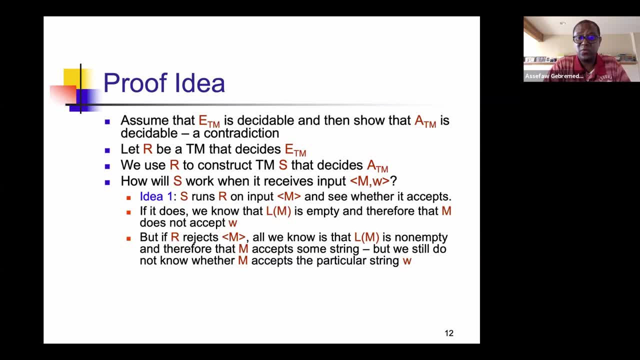 All we know is that this language is now non-empty. We don't know whether it is, and therefore it means it accepts some string, But we still don't know whether M is going to accept that particular string And therefore we don't know whether M is going to accept. 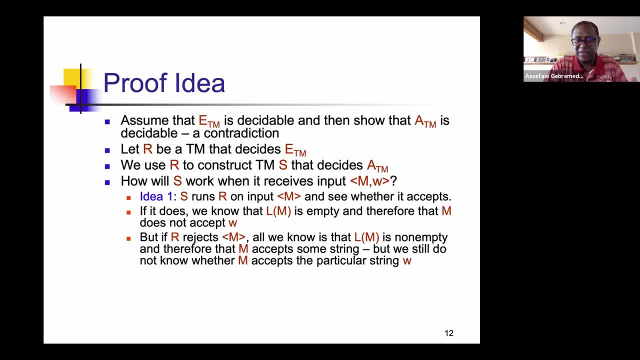 that particular string W, And this is the place where you would learn some tricks, And so this basic idea of how to prove reducibility using contradiction and so on. by now you have believed me, And so you've seen examples. What you will build on more as you learn a little bit more. 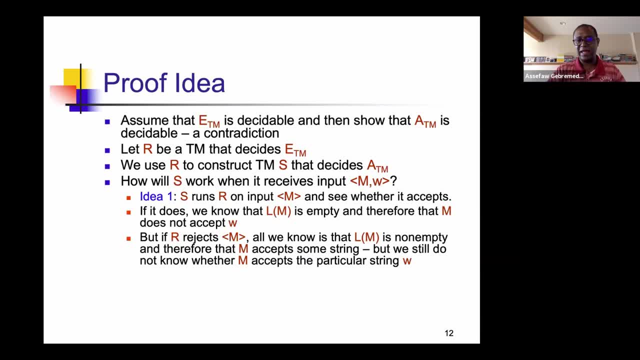 now and as you do, more exercises will be to have some tricks. some tricks where you will say: OK, this is that work, And then I'm going to tweak it this way, I'm going to fix it this way, so that the reduction 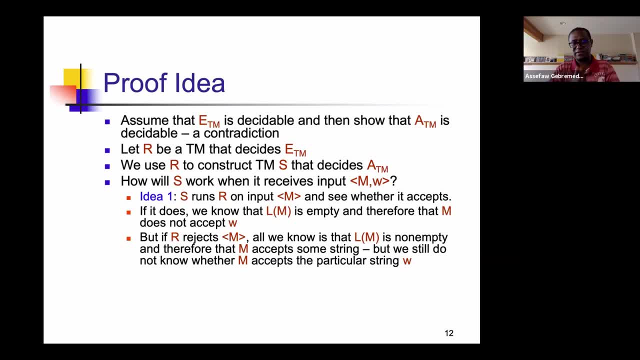 will be successfully done. So this first idea that came didn't work. because it just didn't work, It just told us half the story. So we know that this thing is non-empty, but we don't know whether W is going to be accepted. 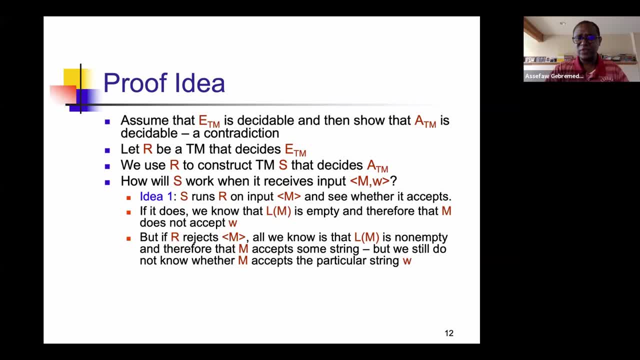 And that's exactly what we want to know. That's what ATM was. So the fix is not difficult. We just have to take care of this W, And so we are going to use a different idea that will just do that modification. All right, so this different idea, we'll call it idea 2.. 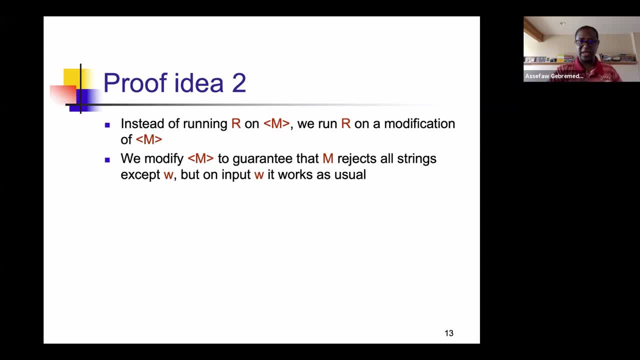 Instead of running R on the machine M, on the encoding of the machine M, we're going to run on a machine. We're going to run a modification of M And the modification is going to guarantee that M rejects all strings, because we 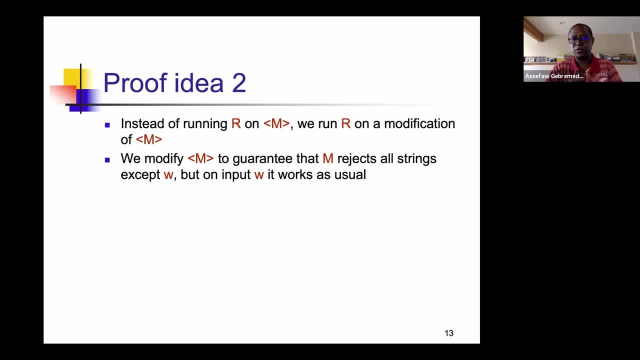 don't care about them, except W. But on input W it works as usual. It will accept or reject, depending on what the W is. Otherwise, for other things we're not going to care because that doesn't matter. 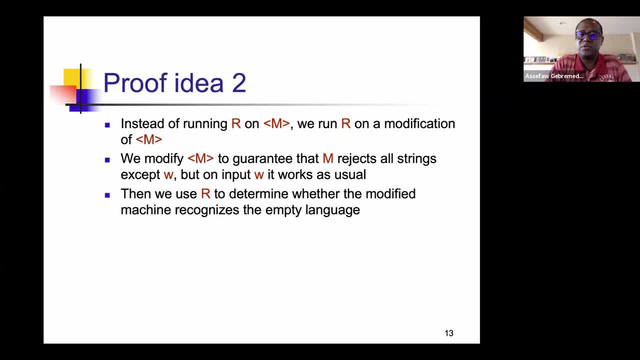 Therefore, then, we are going to use this R to determine whether the modified machine now recognizes the empty language. That was our business. The empty language that we are going to ETM is what we are trying to see, whether it is decidable or not. 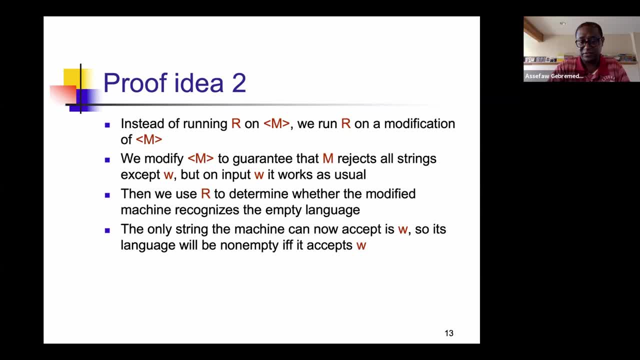 So the only string the machine can now accept, the way we have described, the way we have modified it- is going to be W. So its language will be non-empty if, and only if, it accepts W. So now we have found a one-to-one. 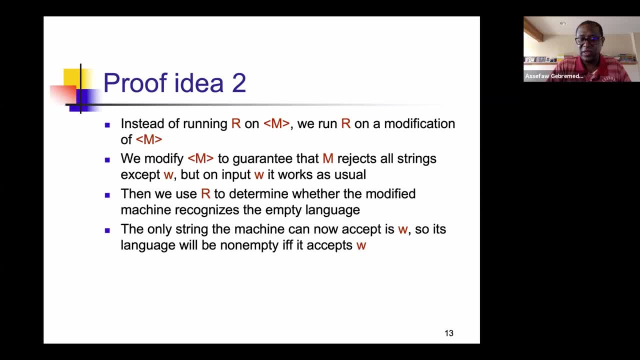 correspondence, whether W is accepted or not, and the empty language If R accepts it. when it is for the description of the modified language, the way we have done now, we know that the modified machine doesn't accept anything and that M doesn't accept W when it accepts. 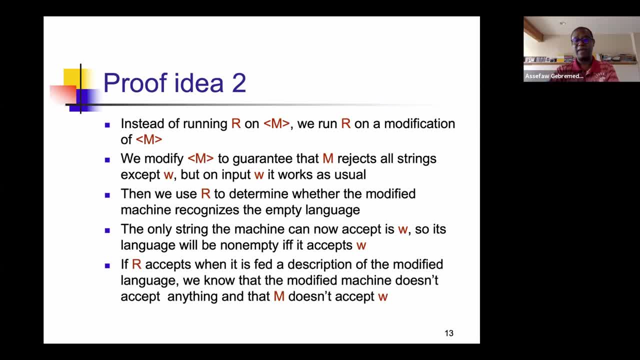 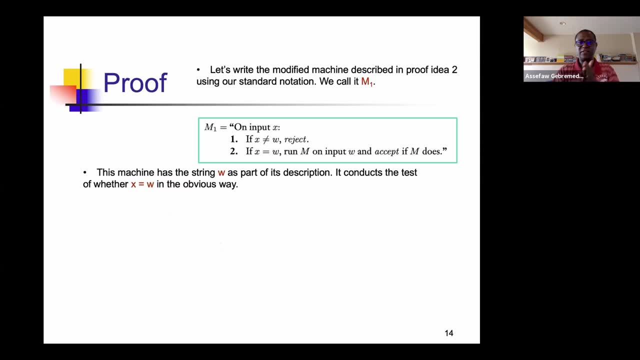 And so this modification now would make us determine whether L M is empty or not, but will it be reduced to whether W is accepted or not? And so here we have the complete proof. now, And because I need a little bit of real estate, 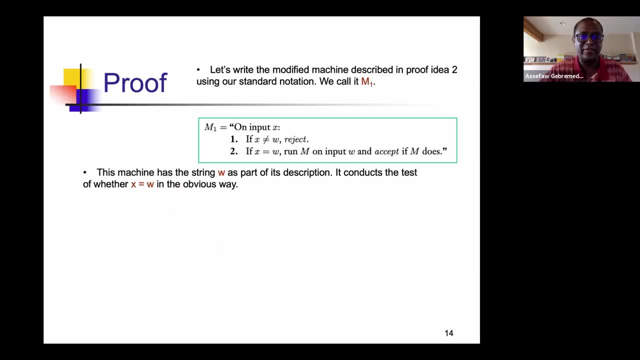 and I have this slide, so I've started to write stuff on the title slide, So that means there is something coming up here. So we're going to have this modified machine which we described in the proof idea tool, and then we're going to turn it into our standard notation. 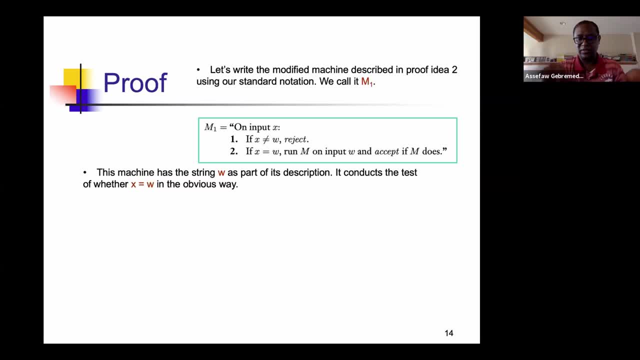 We'll call this one M1.. So we're going to now need, in the formal description, more machines. So we have just this bit that has turned it into accepting just W. We don't care about other things, And so that's supplementary, or that modification. 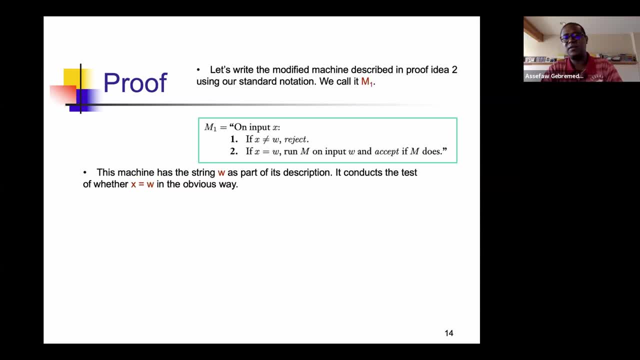 but we're going to call this machine, we will call it M1.. So on input X it's going to say if X is not W, then we just reject, We don't care, If X is W, then we run M on input W and accept if it does. 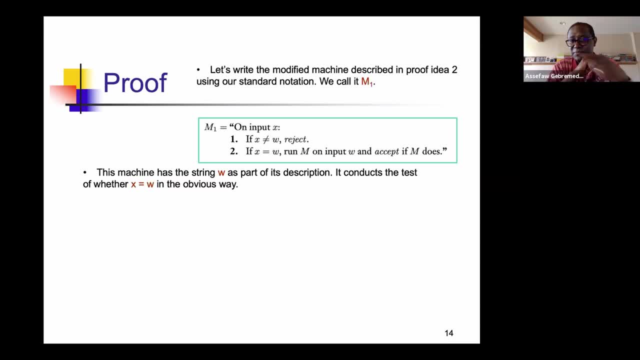 and not if it does not. So that will be what M1 will do. So now we have this machine, M1, has been given an extra task: It's to reject everything else. That means now it has to compare on input X whether it is. 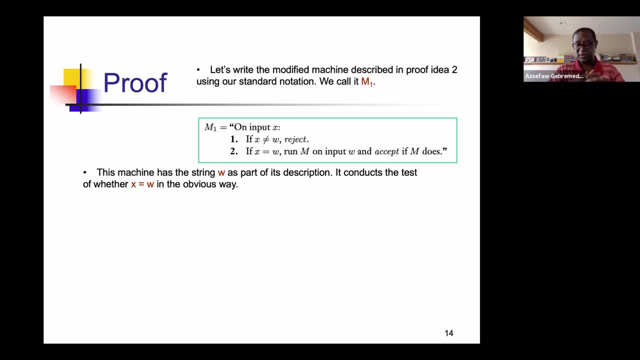 the same thing: It's equal to W or not. So the machine now has got W as part of its description, And so it conducts whether this X is equal to W in the obvious way. By that I mean we will go character by character. 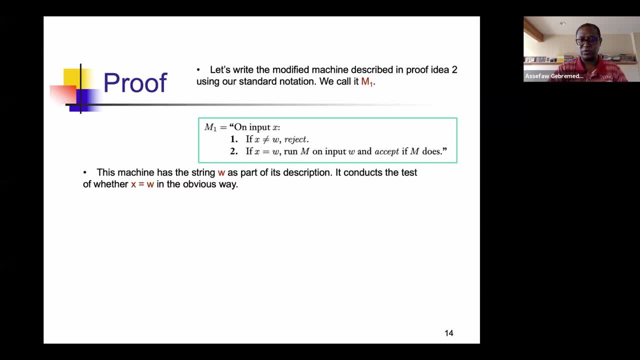 and compare X and W and determine whether one is true or not. So now we have taken care of one piece, the one that would help us with the modification. The rest will be now to use this and describe the Turing machine, R, that besides ETM, and to construct the Turing machine. 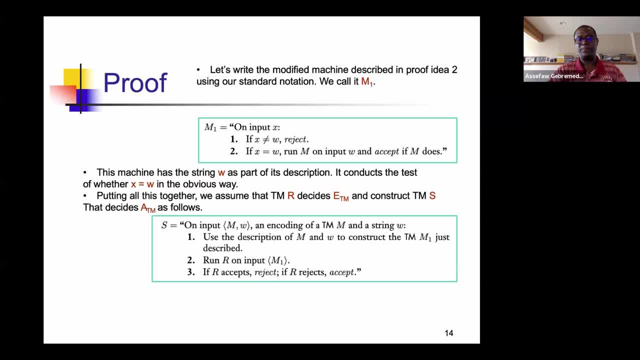 S that besides ATM, And we'll do that in the following way. So we've got S. This is the Turing machine now that is going to decide whether ETM is, or determine whether ETM is decidable or not. So it's going to take on the input. the description of M. 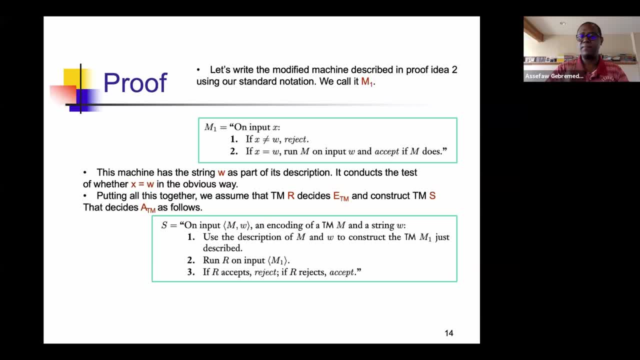 and W, the encoding of the Turing machine M and string W. It's going to use the description of M and W to construct our newly found machine M1, which we just described, And then we're going to run R on input M1.. 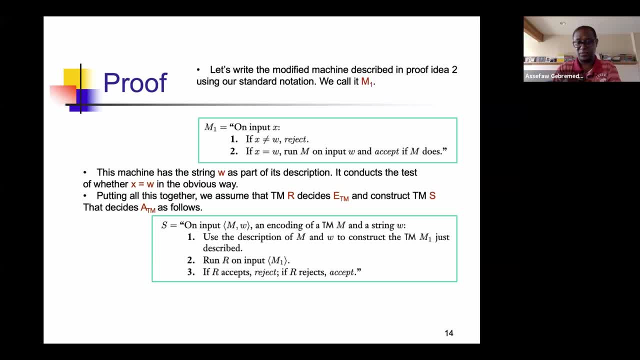 And if R accepts, we reject. If R rejects, we accept. Why are we doing the opposite? Because if it accepts, that means the set is not empty And therefore we reject because ours is about emptiness, And if it rejects, that means it is empty. 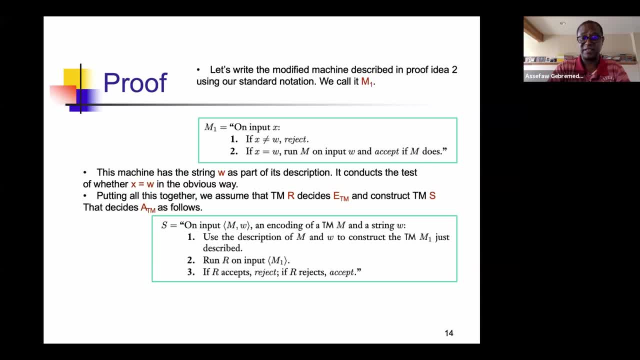 And therefore we would accept. Now, if we do this successfully, then it means if R were decided like this, then S would be a decider for ETM. But we know that ATM cannot exist because a decider for ATM cannot exist, because we have established. 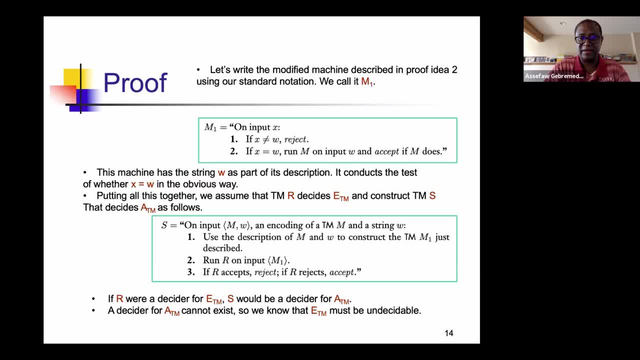 that ATM is undecidable And therefore ETM must be undecidable. So what we have seen in this second example now, the first one was easy to find: the reduction And there was not any new thing that we needed Here. we needed more things to do. 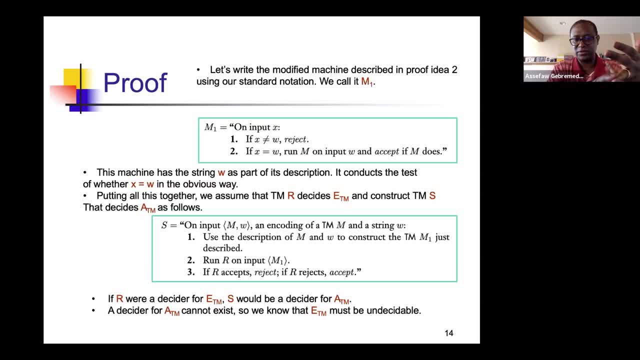 Otherwise, having to arrive at a contradiction, having to do the reduction and then to argue for the fact that if the new machine, if the new language was decidable, then ETM would have been decidable, is exactly the same. So we saw two examples. 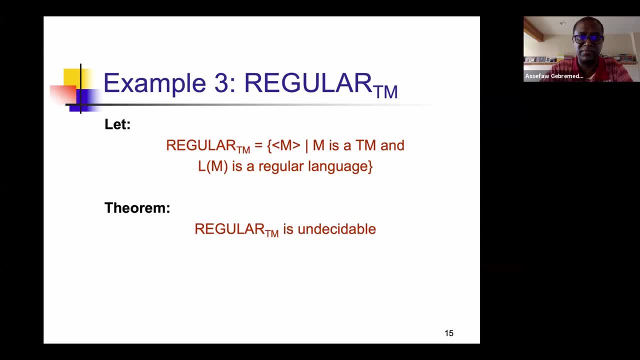 I'm going to pause for a second. As I said, I don't necessarily have a big intention of just having to go through all of the examples, But let me pause for a second and see if anyone has got any questions. how much you're following me. 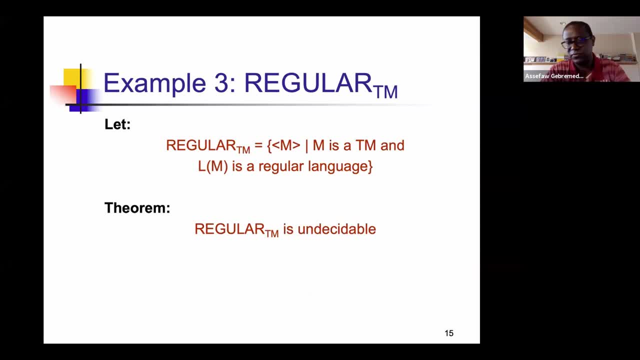 So we've got 10 minutes. So we are. I'm probably able to finish all four examples, Or maybe we'll take one more example. The third example is displayed on the screen, But I don't want to rush, So let me see where you are. 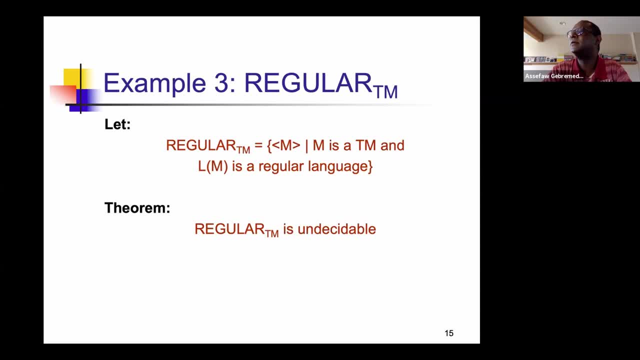 Are you following me? OK, So how should I interpret silence? OK, Thanks, Mostly, I guess. OK, All right, So this is good. So let me, you will get. I think a good way to make through this one would be to see more examples. 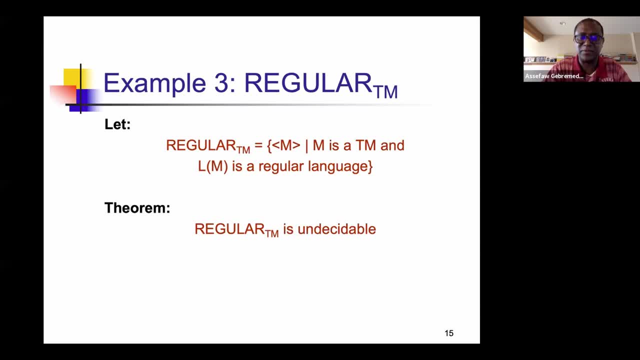 So it doesn't necessarily help to go back through the two examples we have seen so far, But it's not a bad idea to just run mentally And it will give you a break also to think about what has happened so far. What are we doing? 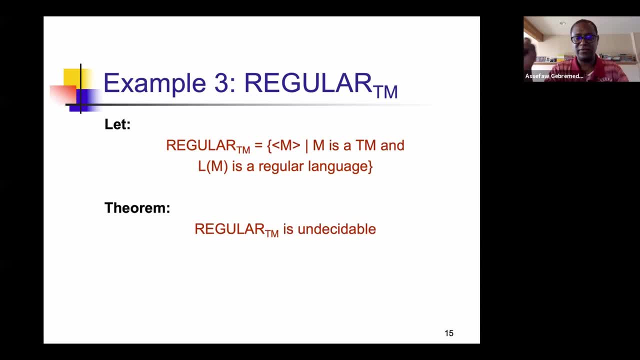 We are in the business of showing things are undecidable. OK, For ATM, we work the hard way. We did diagonalization and showed it. Good, Now we're going to use that one to show when something new comes: is undecidable or not. 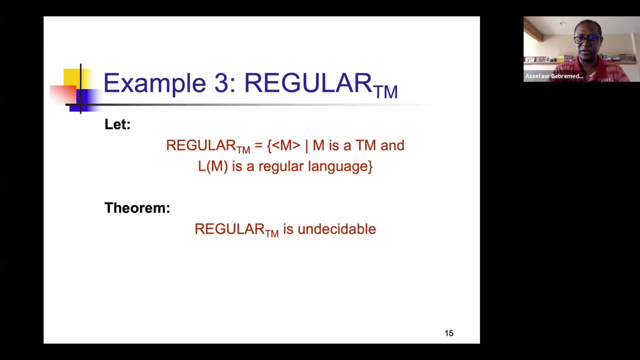 What do we do? We take ATM and reduce it to the thing that we are considering. If this reduction was going to be successfully done and that the new problem was in fact decidable, then the original problem would have been decidable. 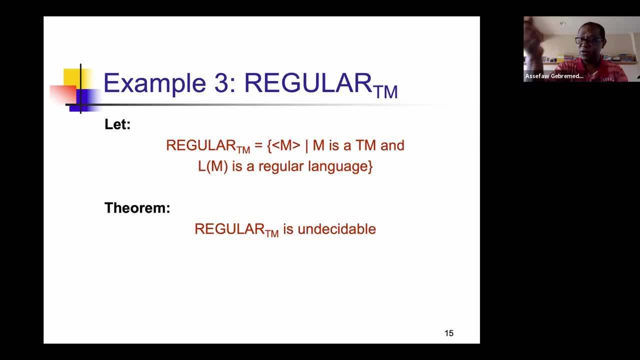 Therefore, after we have shown this reduction, we conclude that the new problem is undecidable. Also, and so that way, we took care of two: Hold to M. Does the Turing machine hold And then empty? Is the Turing machine an empty set? 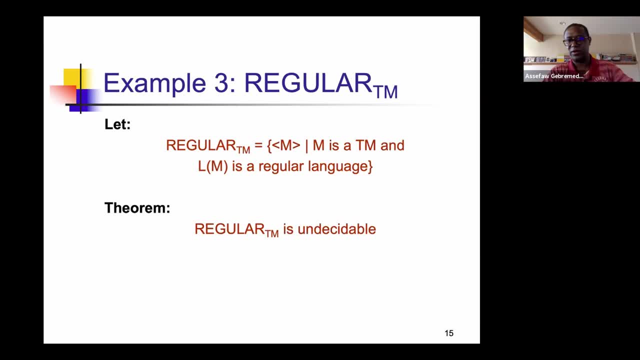 Those problems, if you remember, were decidable when they were context-free grammars. They were when they were regular language, But they are not when they are Turing machine, And that should not surprise you, intrinsically, why that would happen. So we saw two. 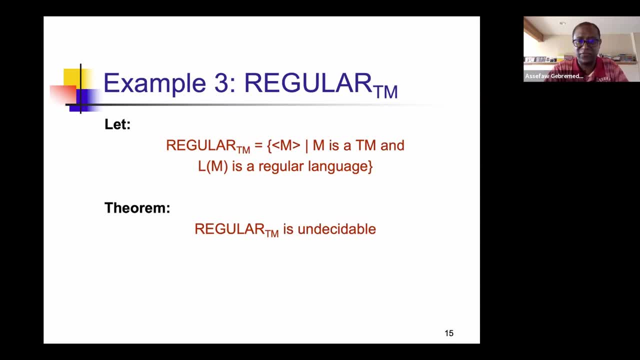 Let's go get another one, the third one. This is going to be fun Because this is actually going to say: if I have a Turing machine, can I have a finite automata that does an equivalent job, as it is Another way of saying it would be. 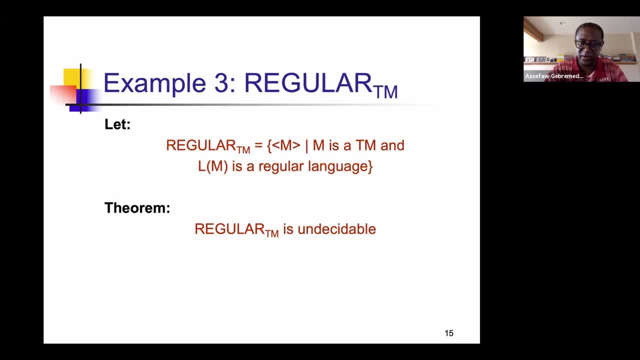 we call those language regular language when there is an NFA or a DFA to describe them or a regular expression to do them. We know this from chapter two. That means now we can have this language called regular TM And it will say: got an encoding of a machine. 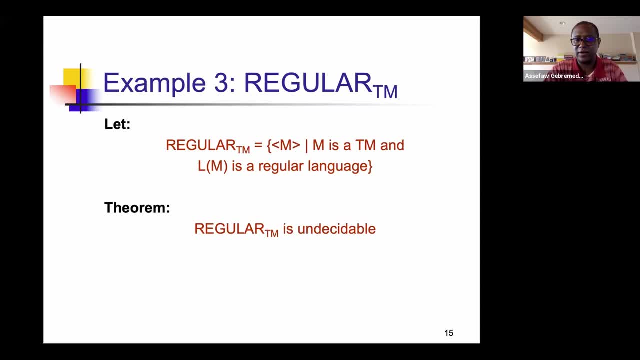 M is a Turing machine And the language of M is a regular language. It might find a bit disappointing to you. This is not decidable, But this is not the only one. Many other ones like this are also undecidable. I'll come back and formulate a nice problem for you. 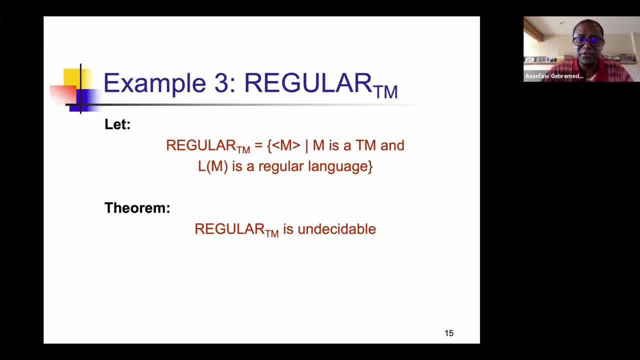 for a homework next time sometime in the future. But regular TM is undecidable. Is there an equivalent NFA or DFA for something that is expressed as a Turing machine? is another way of saying this one A mathematical way and a concise way? 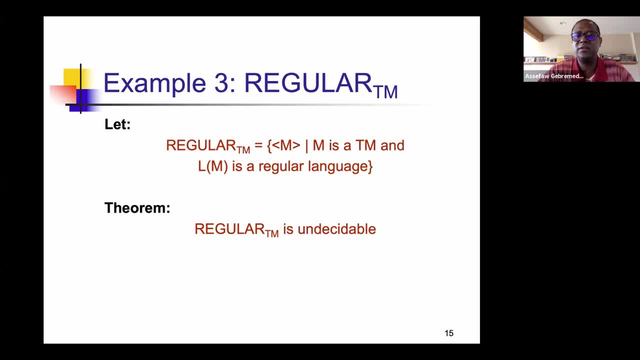 of saying it is what we just have on the slide. now We've got a machine And it's encoding, It's a Turing machine, Either language regular language, Either language of M a regular language, And we can decide that. 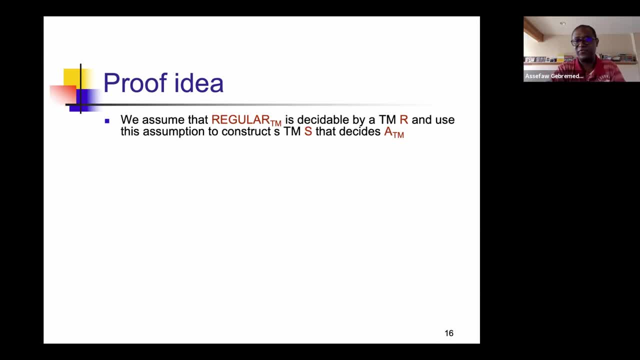 So here is the proof idea We assume, so we have five minutes. If I just run through the proof idea and we don't have the formal proof, I will not worry. We'll pick up next time And I will not hold you more time than you need for this one. 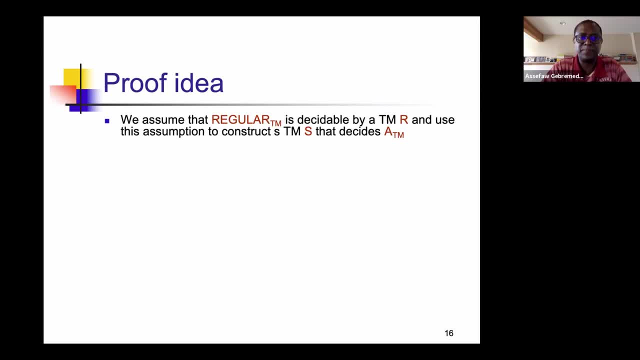 So let's see how far we can go with having to sketch the proof idea. We assume that this Language, regular TM, is decidable by a Turing machine- R- OK, we've seen R so far repeatedly And use this assumption to construct a Turing machine. 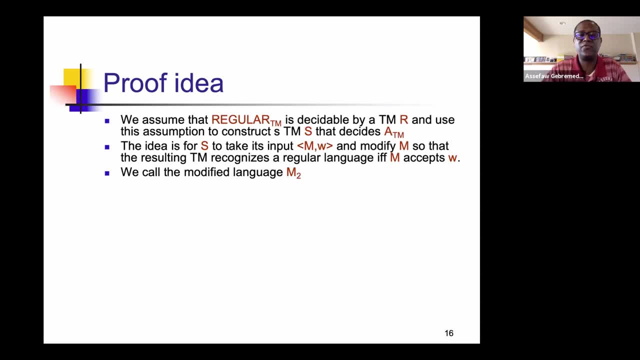 that decides ATM. Fair enough. The idea is for S to take its input MW and modify M so that the resulting Turing machine recognizes a regular language If, and only if, M accepts W. that's also fair enough, And we will now call this modified language M2.. 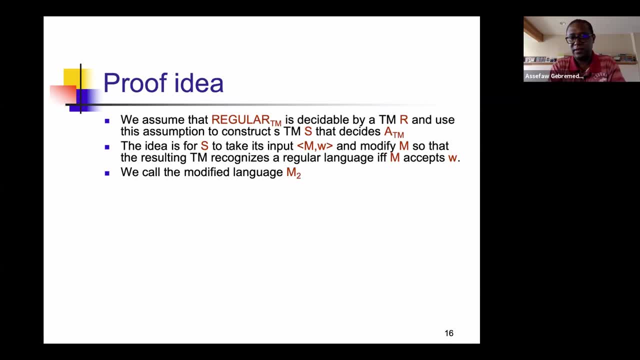 So it will accept If, and only if, the resulting language is a regular language. M accepts W if, and only if, the regular TM recognizes a regular language, And so we'll call this modified language now M2.. And so we are going to now have a design task. 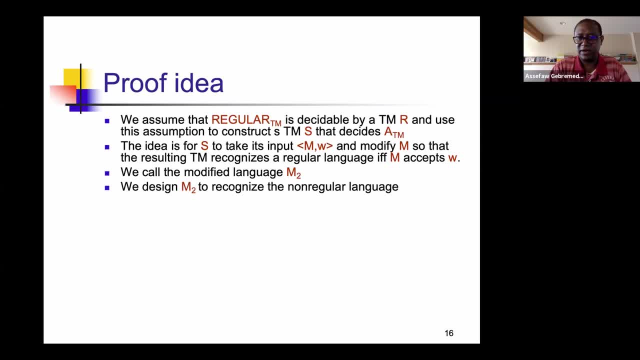 to do about M2, to recognize the non-regular language, And so we are going to be doing this because we know there is at least one language that we know is not regular And we're going to use it to design, And so the name regular language we'll. 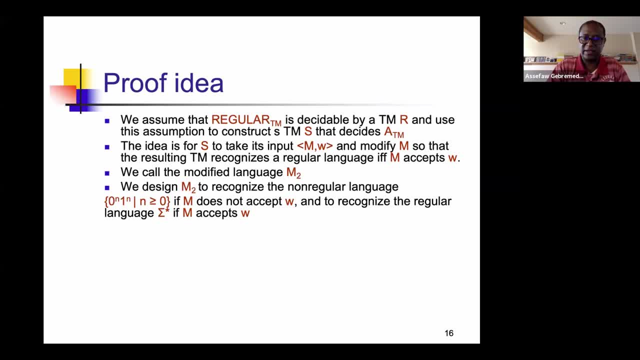 use for this construction is 0 to the N and 1 to the N. We remember this one. This was not regular And we will use this. We will design this machine- the modified M2, to recognize this non-regular language if M does not accept. 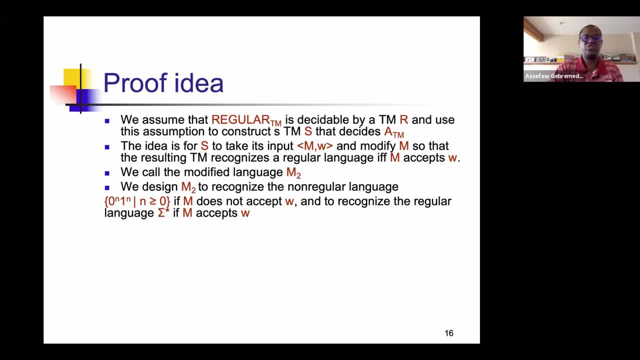 W and to recognize the regular language. that's just everything else if M accepts W. So that's what the input is doing. So now we have done a clever construction. a clever construction by picking up a non-regular language and to use this one if M does not accept W. 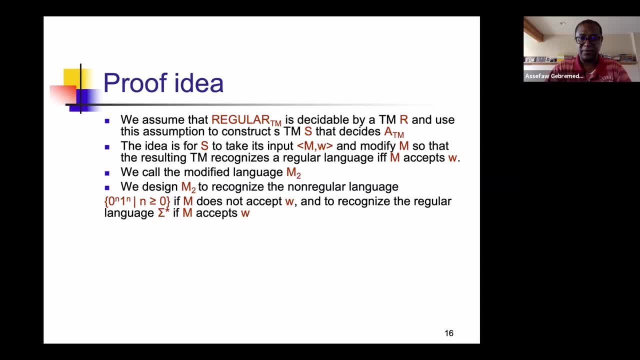 and to use everything else when M accepts W. So this is where the cleverness would come. It may not be something that very intuitively comes to your mind. This would, among other things, would have required us to pick a language that is non-regular. 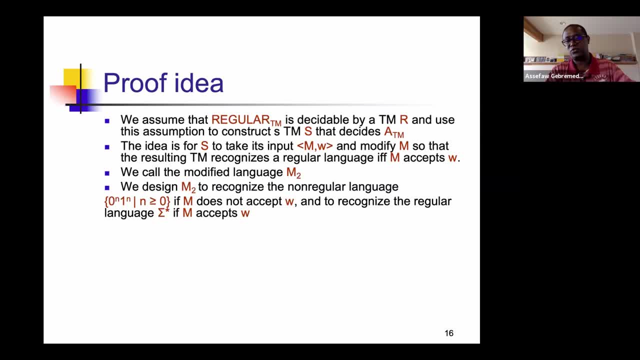 But the idea of having to show this reduction and to argue for the fact that if this was true then you know, ATM would have been decidable, is going to remain. So that's the construction of M2.. And then we must specify now how S can construct such an M2. 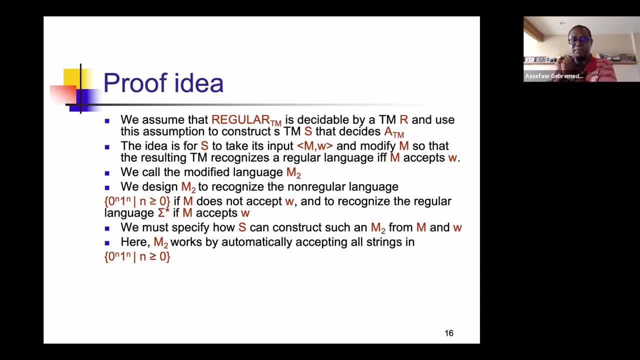 from M and W, And we will do this by making M2 work automatically, accepting all the strings in this And, in addition, it accepts W. If M accepts W, M2 accepts all other strings. So what I wrote in the first bullet. 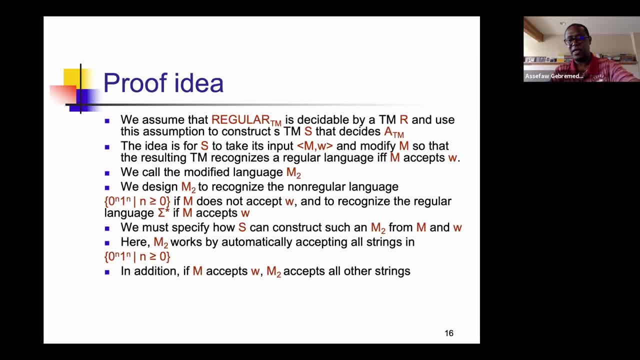 is now what is being added. So there is a little bit of So. there is a little bit of So there is a little bit of A point that you will probably want to think about on this one, And that's probably a good point to stop. 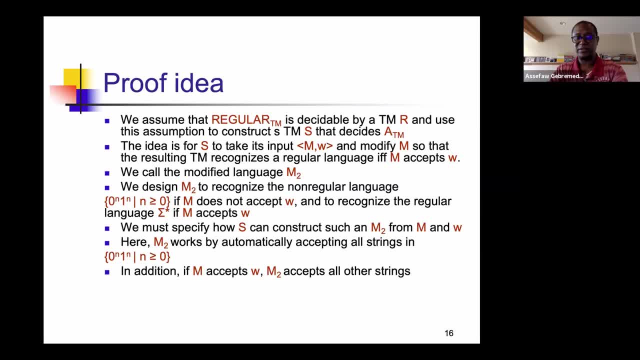 And then, when we start next time, to pick up. But this is where the idea, the construction of this proof, is going to go forward. So, as I said, I don't have any problems stopping at this and picking up from what we have. 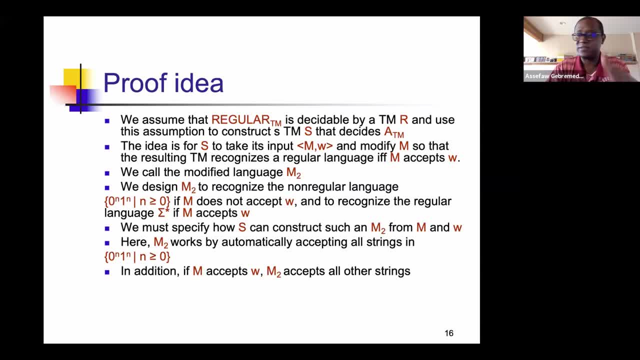 We have done- at least successfully- two examples, So we'll see more examples next time, on Wednesday, And I think I will probably stop here. I'll have one or two more slides when I post them on, as well than what we are just seeing here.